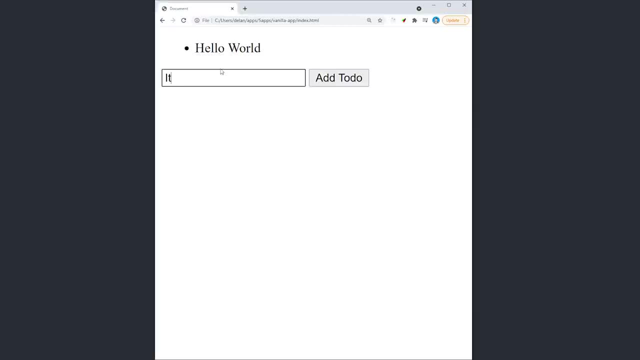 then add a script tag to the body. What we want to build here is a to-do app where the user can write some text into a form input, then submit the form and have that item appear in the list. In addition, we'll save those items to local. 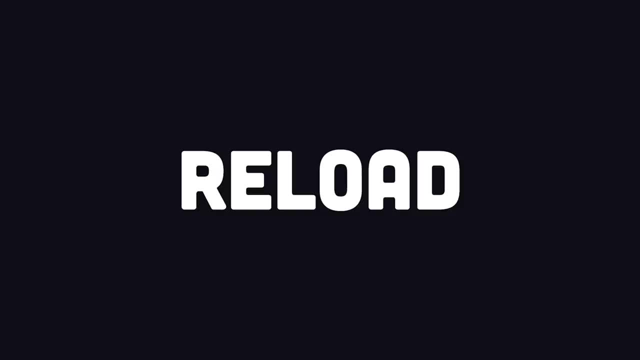 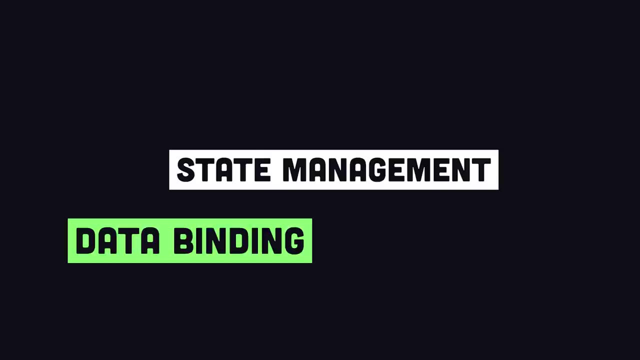 storage as kind of a mock database so that when the user refreshes the page those items are still present. Pretty simple concept, but there's actually a lot going on there, like state management, data, binding events and the application lifecycle. to think about The 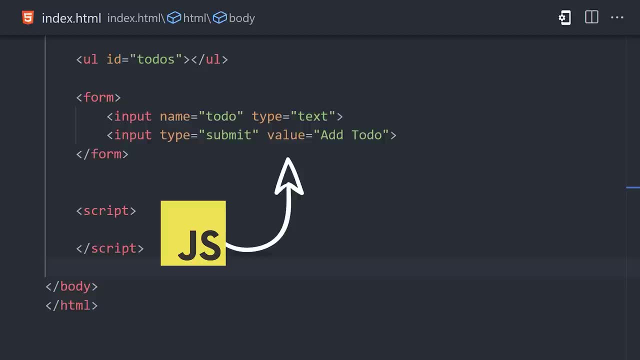 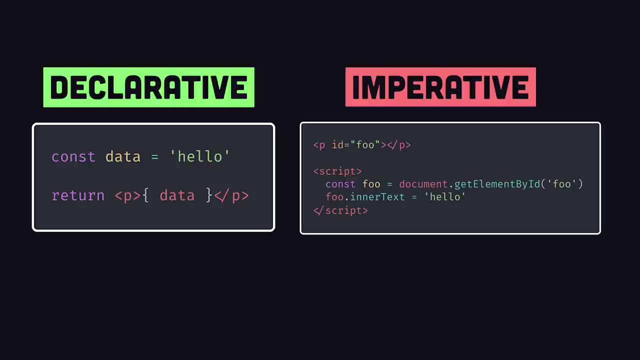 one thing that all frameworks do, and vanilla JS doesn't, is provide a way to bind or connect your HTML to the JavaScript automatically. In vanilla, we need to imperatively grab the HTML elements that we're working with from the DOM, And I can tell you right now this is a very annoying way. 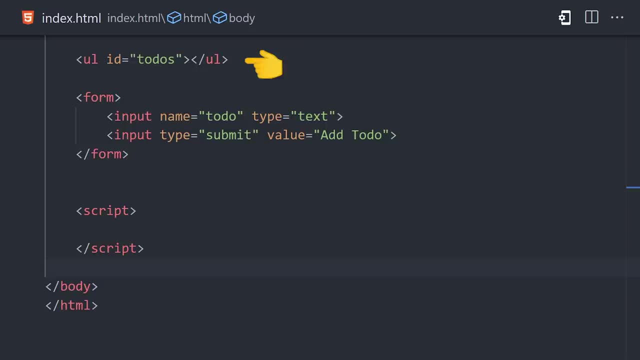 to build a complex application. As you can see, here in the DOM we have an unordered list for the to-dos and then below that we have a form with an input and a button to submit the form. Now, going into the JavaScript, the first thing I'll do is write some code using document query. 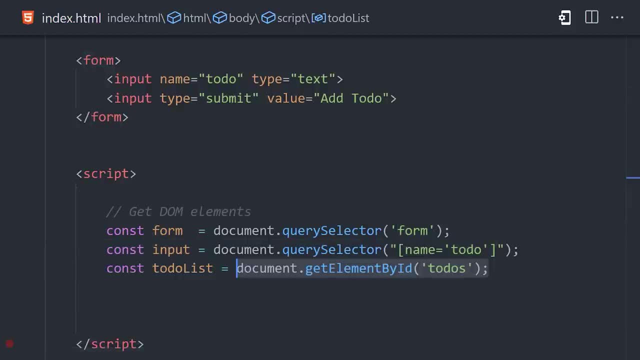 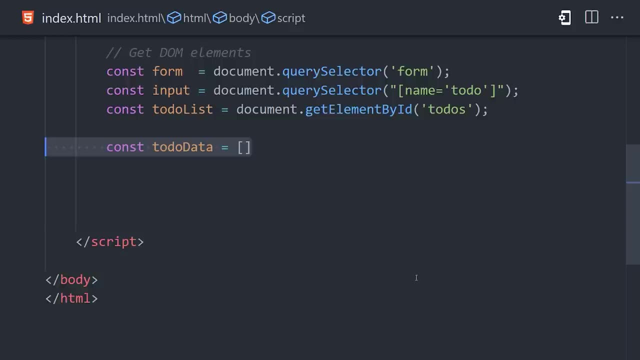 selector to grab each one of these items from the DOM. Now that we have access to the HTML elements, I'm setting up an empty array here to represent the actual to-do items in the list. In addition to keeping track of the data, we also need to update the actual UI when that data 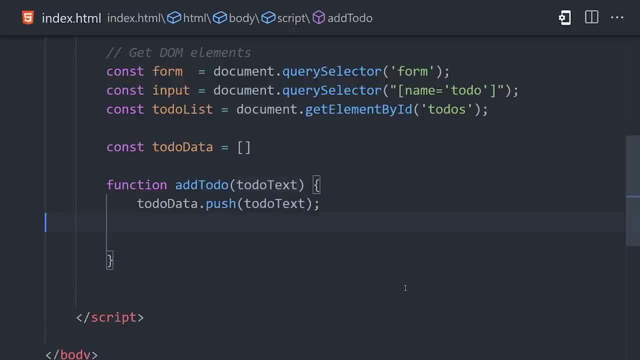 changes. For that I'm defining a function called add to-do that takes a new to-do item as its argument. Now this is where things start to get ugly with vanilla. In order to update the UI, we need to manually create a new list item element by calling document create element. 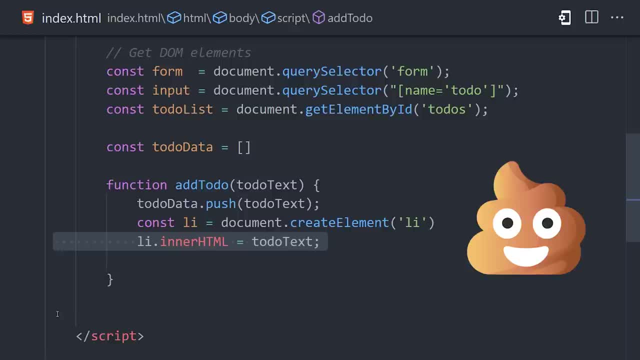 Then we need to imperatively update its inner HTML to the to-do text and finally append it to the unordered list in the DOM And, as an added touch, I'll save the data to local storage so we can access it when the page is refreshed. The problem with this code? 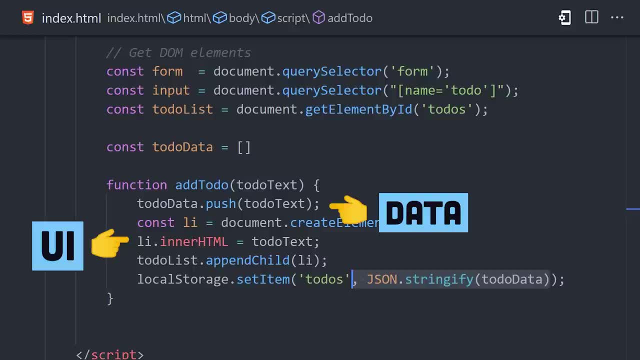 is that the application, data or state is completely decoupled from the UI itself, and that makes it very hard to keep the data in sync with the UI. Now that we have this function in place, we need a way to call it when the user submits the form. For that we need to register an. 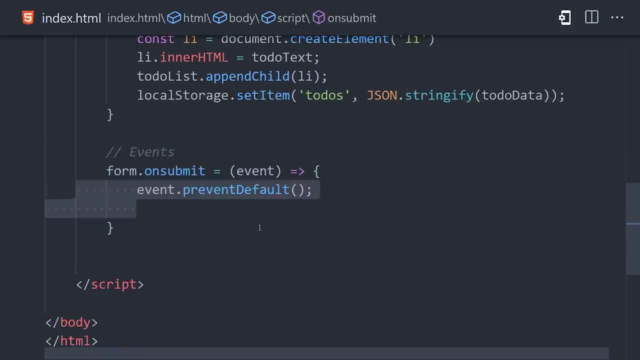 event listener on the forms on submit event. When that event is fired, we'll first call prevent default to prevent it from refreshing the page, then call the add to-do function with the current value in the form And then we'll call the add to-do function with the current value in the form. 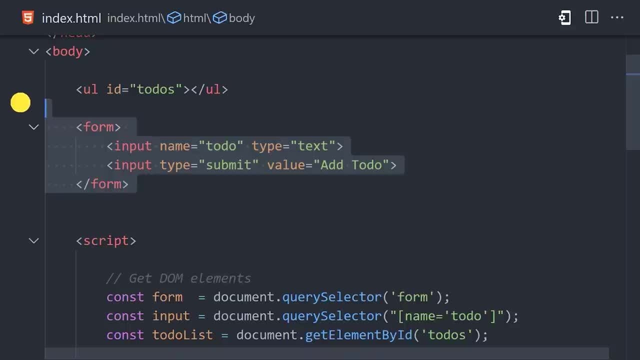 At this point we should have a working to-do list. but one important thing to notice here is that if you look at the HTML markup, you really have no idea what it's doing. There's no way to tell this form has an event listener attached to it, unless you go search. 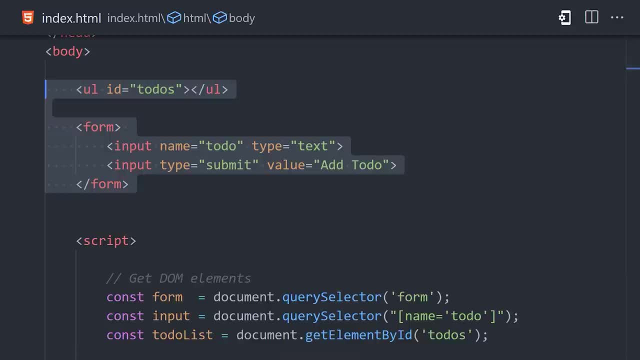 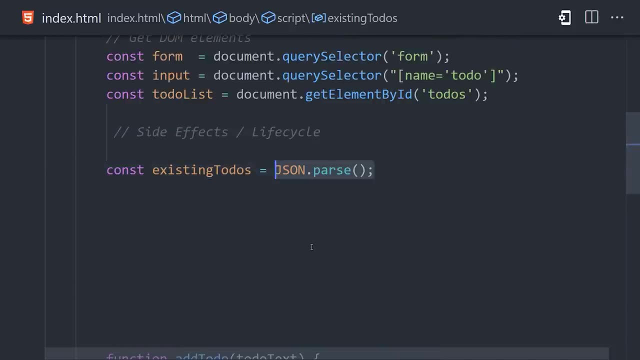 through the JavaScript code itself, which is extremely difficult in a complex application. Now, one final thing to think about is the application lifecycle. When the app is first initialized, what we want to do here is grab the existing to-do items from the local storage. 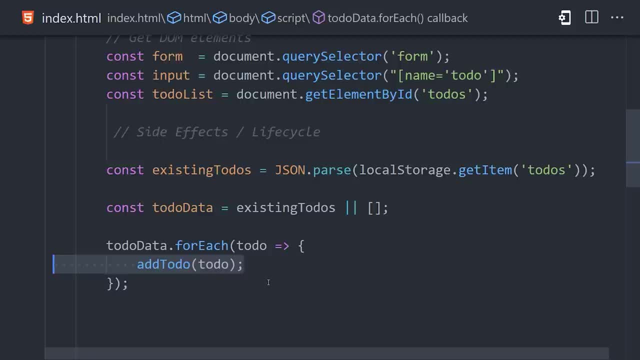 and render them in the to-do list, if they exist. If there are existing to-do items in local storage, we can loop over them with for each and call the add to-do function for each one of them. Congratulations, you just built a to-do app with vanilla JS, But this code is not going. 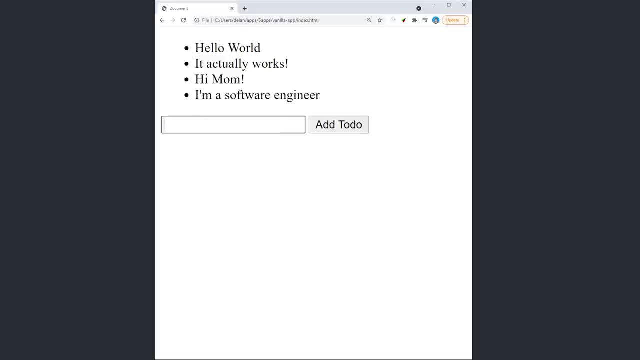 to scale complexity very well, And there's likely many other features we'd want to add, like routing or animation, that we'd have to implement from scratch, And that's why the vast majority of developers choose to build their apps with a framework. First we have React, which most 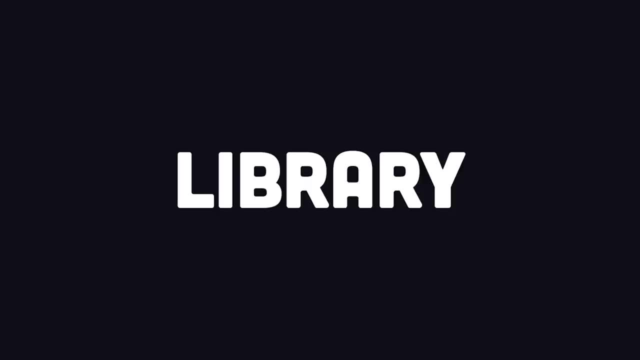 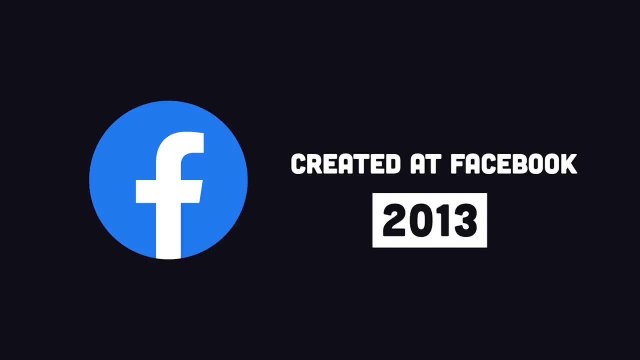 people would consider the most popular framework. Some people call it a library, but it doesn't really matter, because it's a tool that becomes the main driver of your application And that's just another project requiring you, the developer, to do everything the React way. I don't mean that. 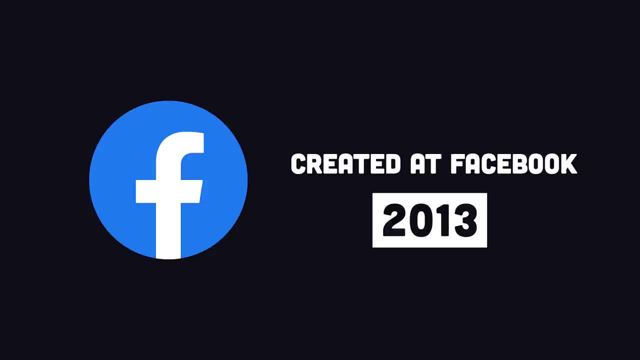 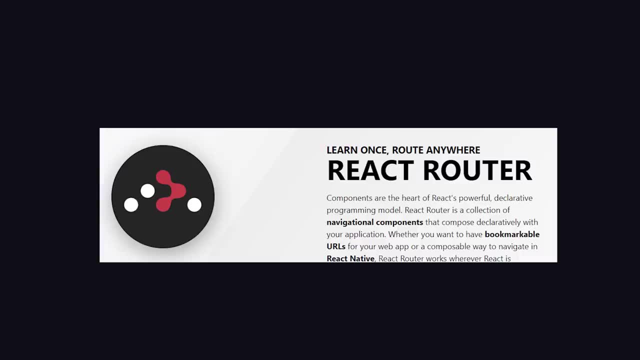 in a bad way because React was created by very smart people at Facebook to build complex UIs like the Facebook UI. React is minimal by design and relies on the open source community to handle other concerns like routing, animation, state management and so on. It's not opinionated about. 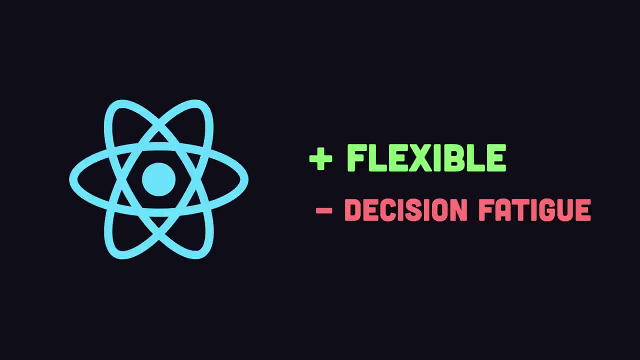 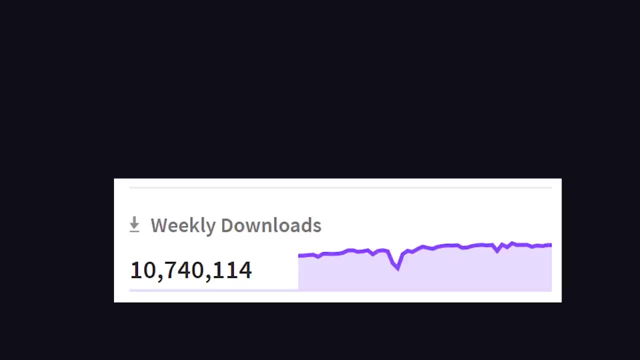 how you organize your code, which requires you to make a lot of decisions about which libraries to bring in and how to make things maintainable and scalable. React is by far the most popular framework, with over 10 million weekly downloads on NPM and over 170,000 GitHub stars. Its popularity. 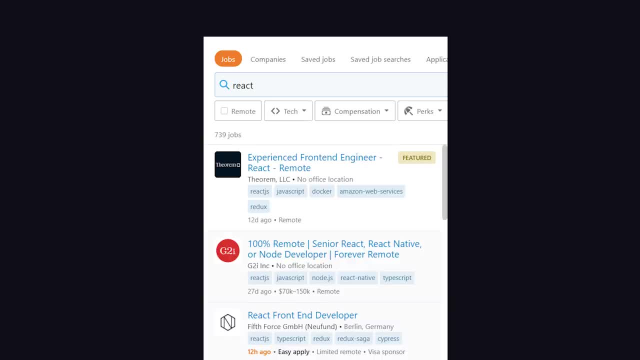 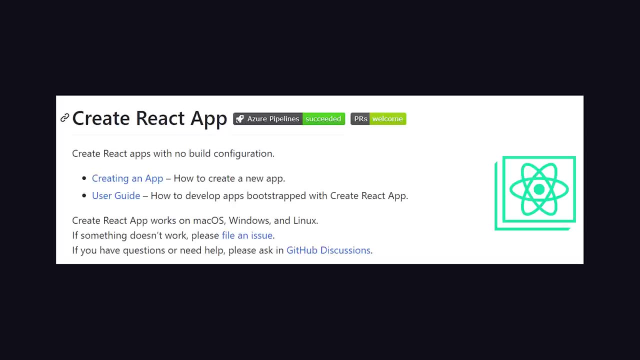 alone makes it a great skill to learn, because there are many employers out there looking to hire React developers, And you'll find tons of other React developers in the industry to collaborate with. React has an official CLI called create-react-app. We can create a new. 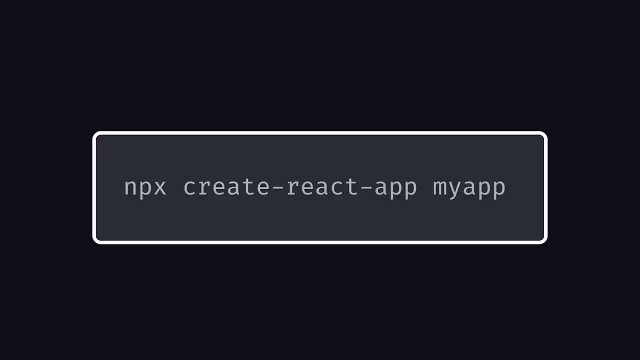 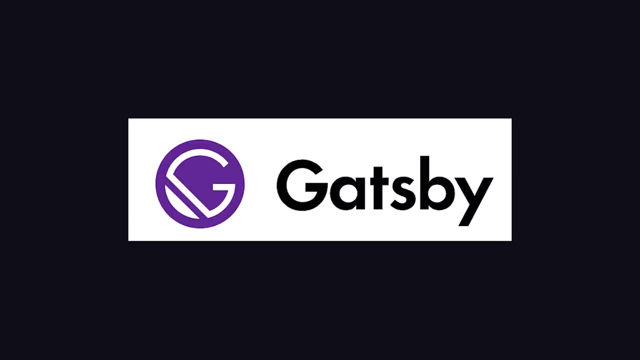 React project by running the create-react-app command from the terminal. Now it's worth noting that many people opt for other tools when building a React project, like Nextjs or Gatsby. that would default CLI. When you generate a new project with create-react-app, you'll notice it has a package. 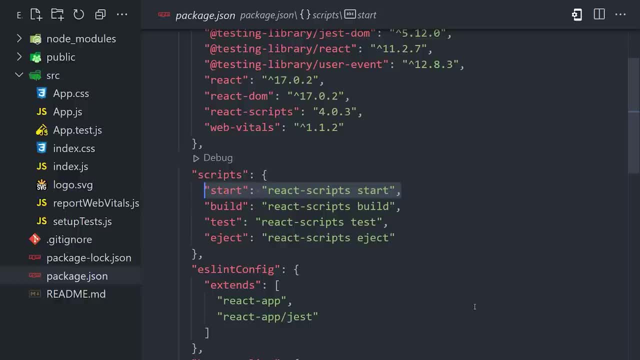 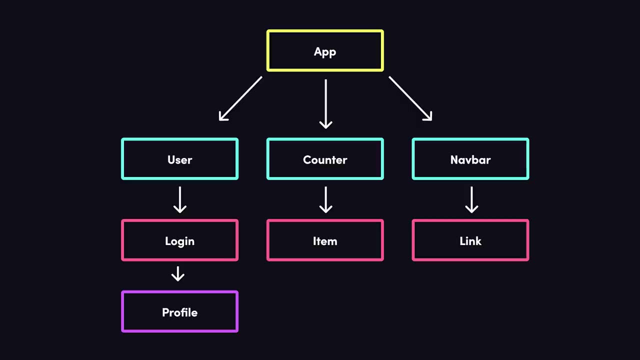 JSON in the root of the project, inside of which there's a start script to serve the app. locally Under the hood, it uses a tool called webpack to bundle all your code together into a single JavaScript file. In React and most other frameworks, your application is organized as a tree of 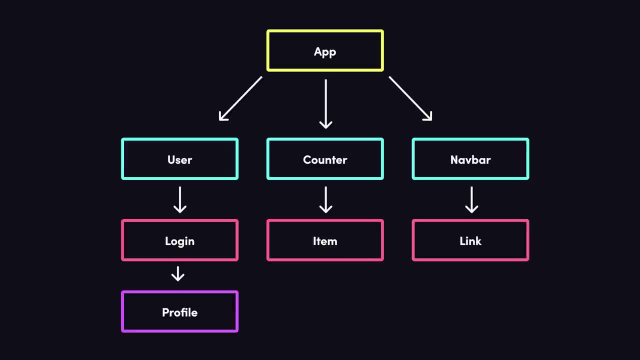 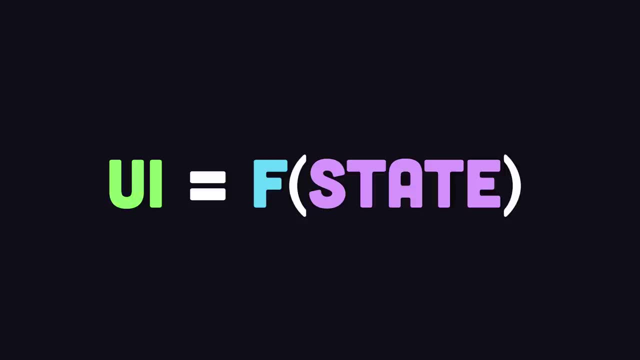 components. These components encapsulate parts of the UI and have ways to communicate with each other. This allows you to organize your app in a declarative way where, for a given set of application, the UI will always be the same. Now, in the appjs file, you'll first notice a function called app. 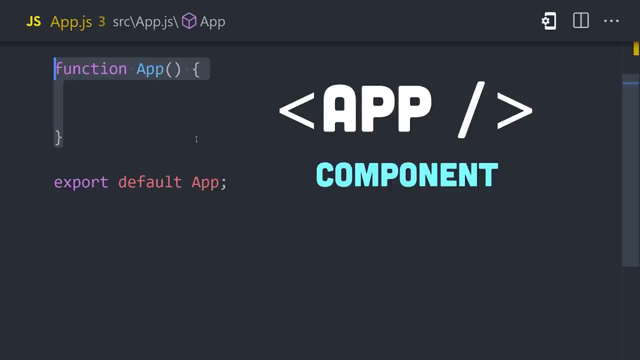 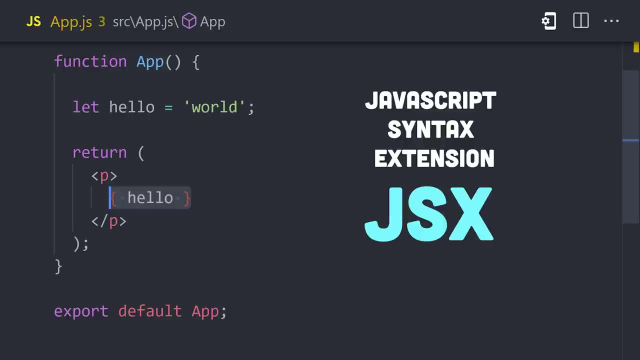 That function represents a component in the UI, And personally I love the simplicity of that. Now the return value of the function is jsx, which itself looks like HTML, but has been extended with an additional syntax allowing you to insert JavaScript into your HTML For the to-do list. 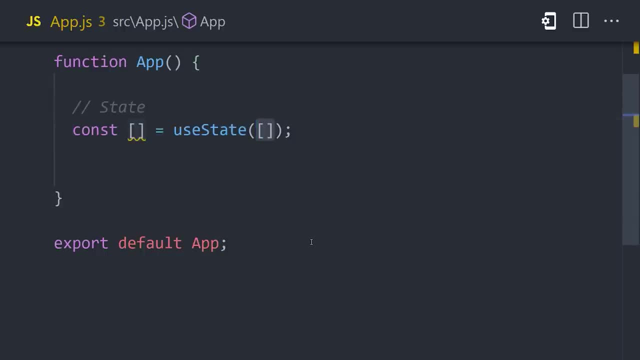 we can define reactive state on the component with the useState hook. The hook is just a function that will show the state of the list. The second item is the value of the to-do list as reactive state, which means anytime it's updated, the UI will re-render to show the latest state And then 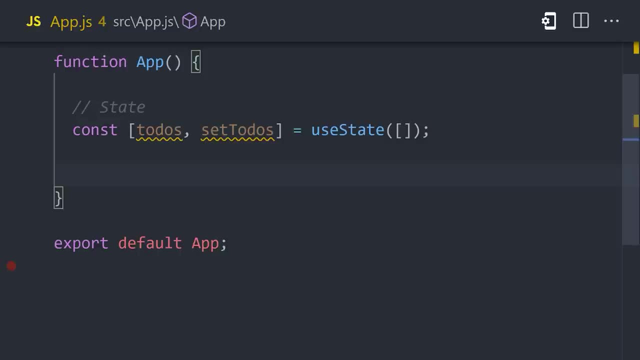 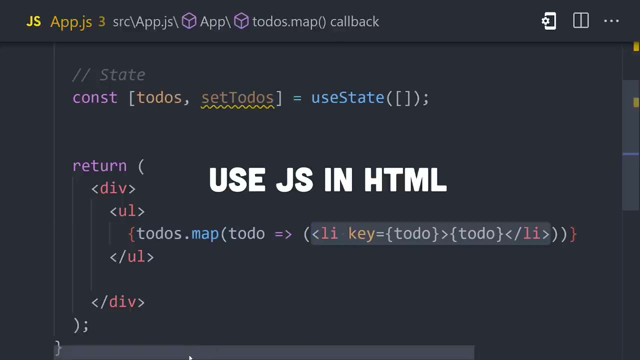 the second item is a function to update the state. Now, if we go back down to the jsx, we can loop over the to-do items in the array and render them out directly in the UI as a list item. Then below that we have an HTML form. But the cool thing about React is that we can bind an event directly to. 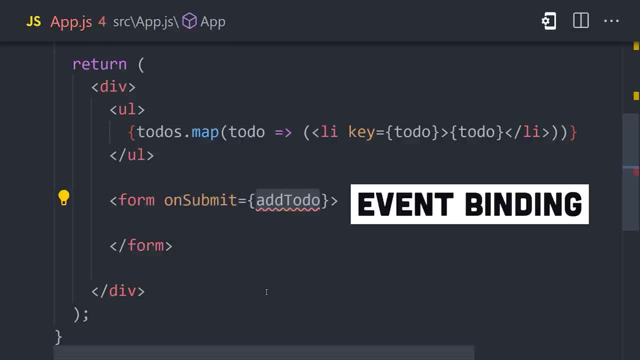 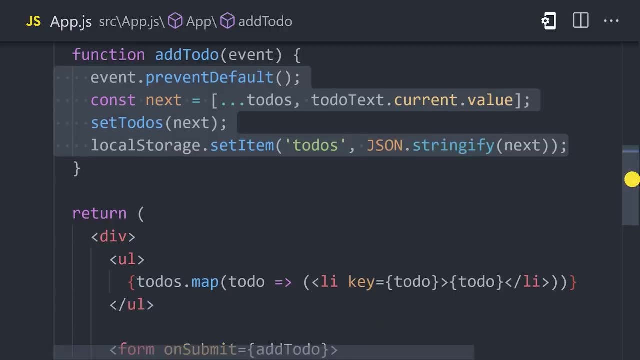 this form using onSubmit. Then on the right side of it we can reference a function that will be called whenever the submit event fires And that function will update the state and store the result and local storage. You'll also notice that I'm using the useref hook to grab the current value. 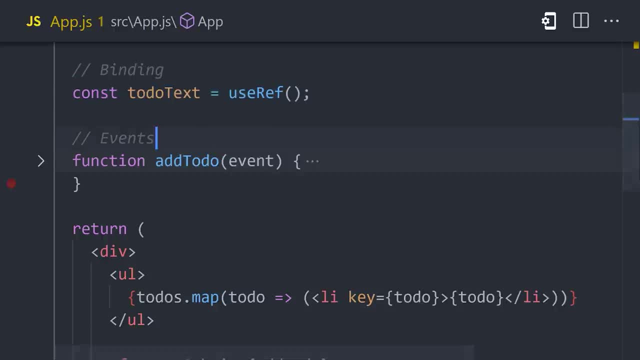 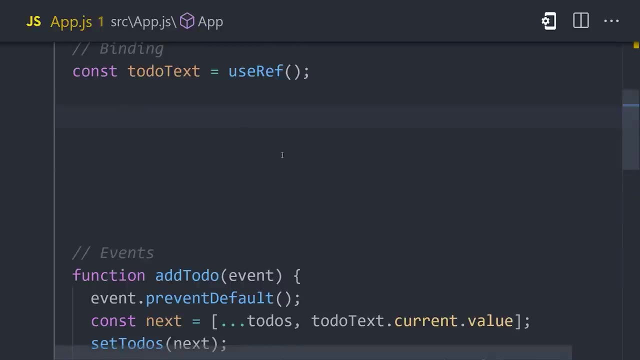 of the form input. One thing to notice here is that the HTML is a lot more descriptive. We know exactly which elements our data and events are bound to. Now, the final thing we need to do here is run a lifecycle hook In React that can be handled with the useEffect hook, which will grab. 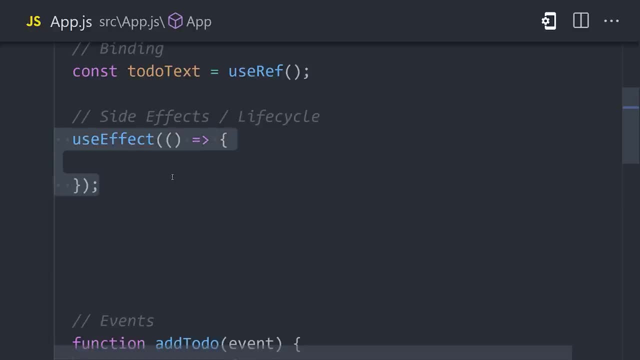 the items from local storage when the component is first initialized. This hook can be really confusing, though, if you're just getting started. To only run it when the component is first initialized, I need to add an array as the second argument, And in my opinion, this code is just. 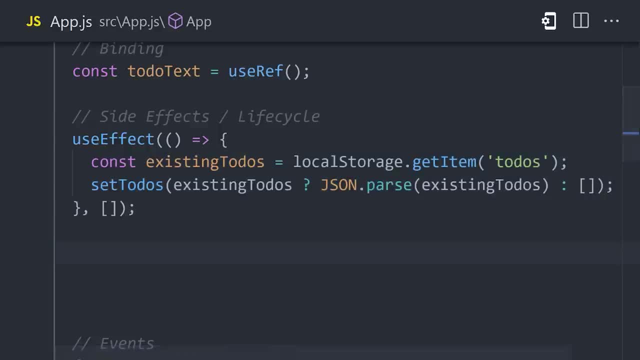 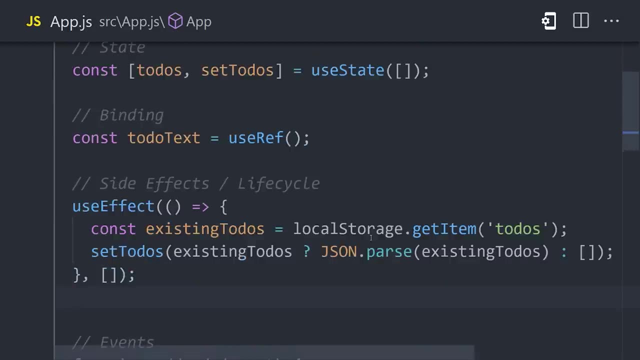 really hard to look at, unless you really know what's going on with the useEffect hook. In any case, React is the gold standard for declarative UI frameworks, But there's more than one way to get the job done. Next we have React's arch nemesis, Angular, which is developed and maintained by Google. 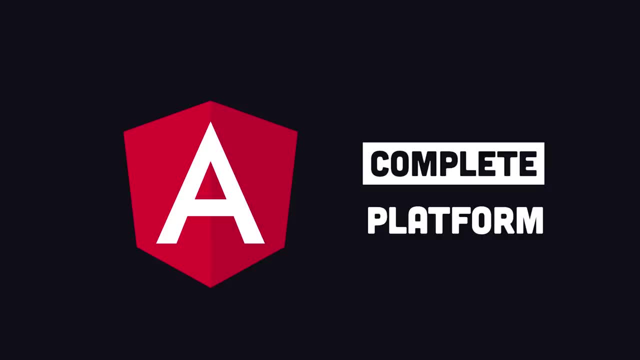 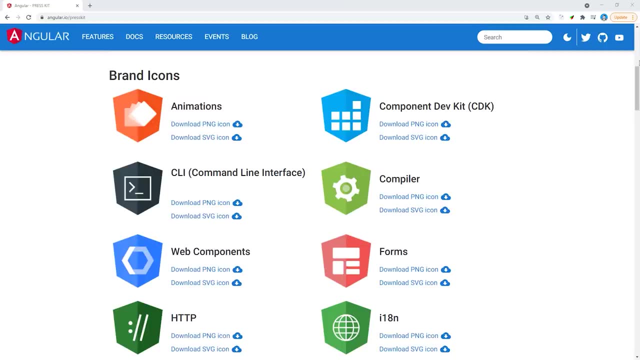 and, unlike React, is very opinionated about how to organize and structure a project. It has 75,000 nodes and is the second most downloaded framework on NPM. It comes with officially supported libraries for routing, animation and server-side rendering, And because it follows a set of 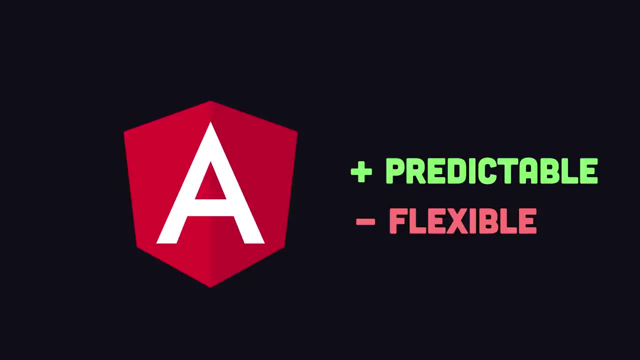 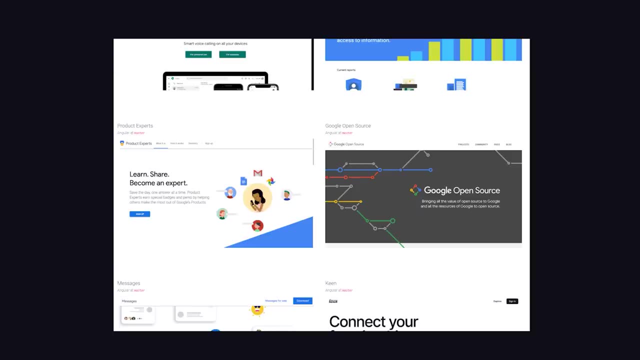 predictable conventions. all Angular projects are structured relatively the same and have awesome tooling to go along with them. In fact, you are actually required to use TypeScript. Google uses it internally to build hundreds of different web apps throughout their product line. It's a. 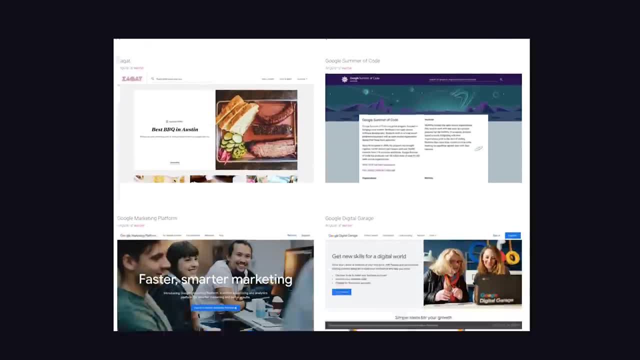 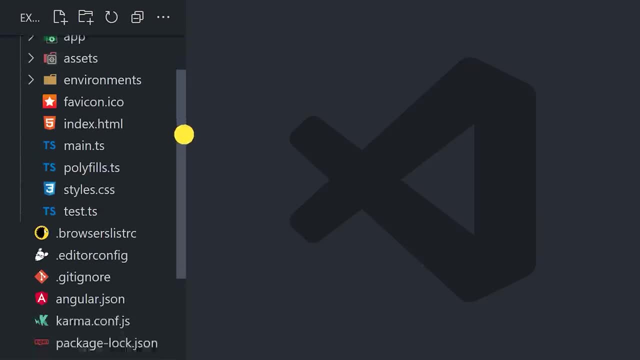 great option for big teams but may be a little overwhelming if you're a beginner. To start an Angular project, run ng new from the command line. That'll give us a fairly large project to build that's already configured with TypeScript. We can build a component in the app-componentts file. 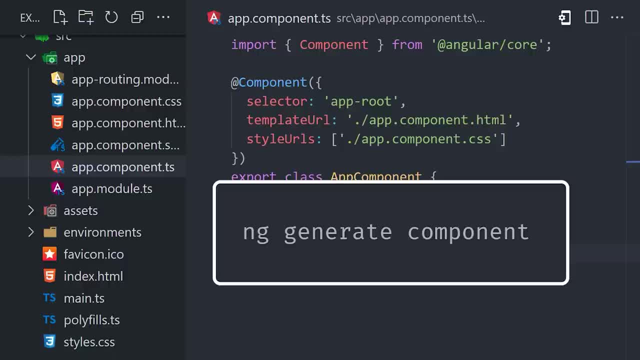 or we could use the CLI to generate a brand new component automatically. In fact, Angular has the most powerful CLI of all the frameworks by a pretty wide margin, And you'll notice the component itself is represented as a TypeScript class that has a component decorator. 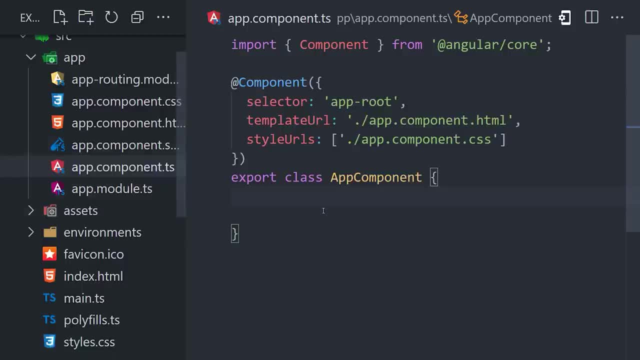 on top of it. Now it is possible to define an entire component in this TS file. However, most Angular apps break components down into at least three separate files: one for your TypeScript HTML and another for the CSS. To add reactive state to the component, simply define a property. 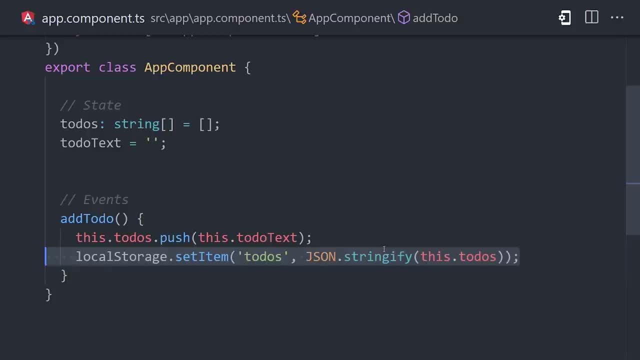 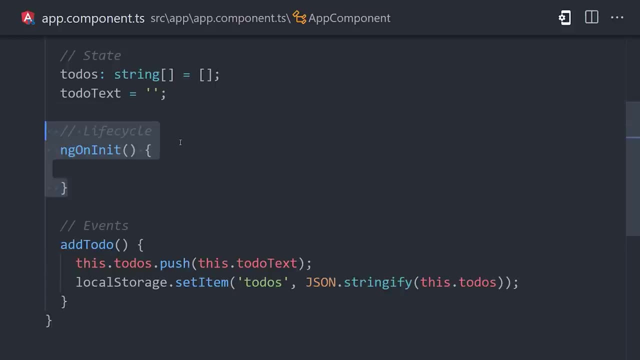 on the class. From there, we can define a method on the class to update the state. In addition, we can manage the lifecycle of the component in the class by implementing special methods like ngOnInit. This method will be called whenever that component is first initialized Now. 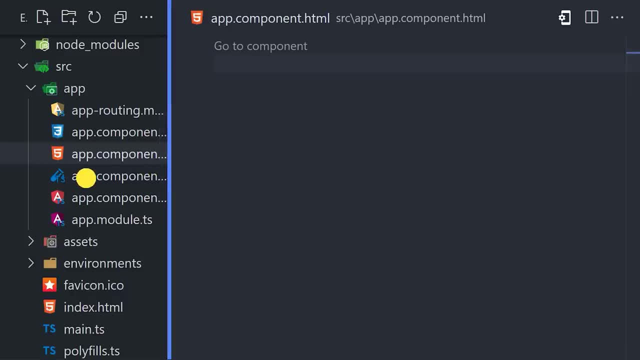 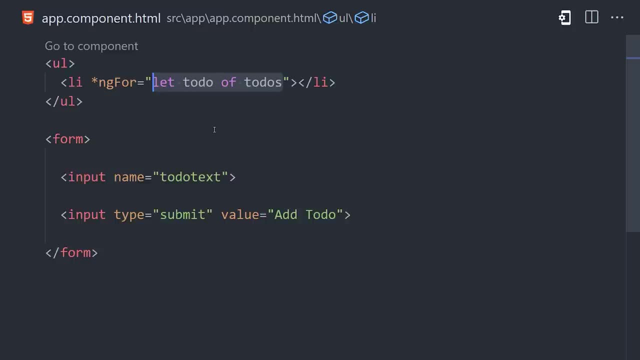 if we go into the template, you'll notice this looks like HTML, but it's been extended or empowered with a special templating language that makes it possible to loop over an array of items using the ngFor directive, Unlike React, which brings HTML into your JavaScript. 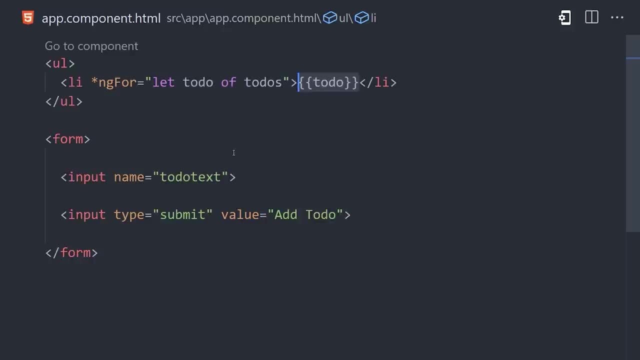 Angular does the opposite and brings JavaScript into your HTML. Then in the form itself we can bind to the submit event and run the add to do method whenever that event is fired. Then to get the actual value from the form input we can use two-way data binding using the ngModel. 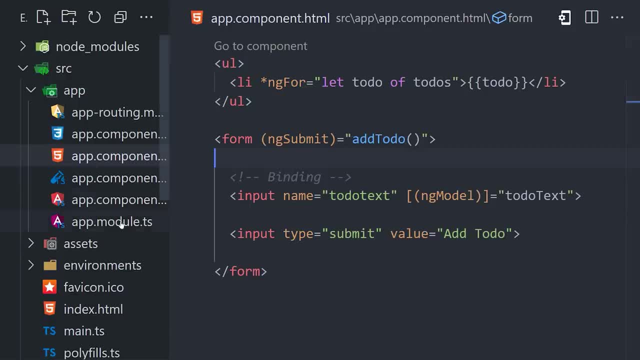 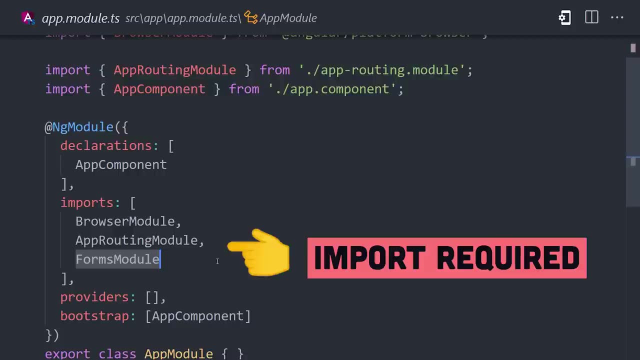 directive. This binds the form value to the to do text property on the class. However, to use this, we need to go into the app module and import the Angular module there, because it's required for that directive to work And for that reason, 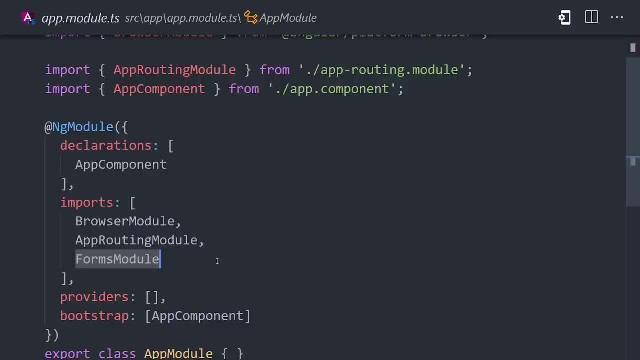 among many others. it tends to have a much higher learning curve than other frameworks, But everything is here for a reason, and Angular is very opinionated about how to structure a project that will scale well And that tends to make it very popular with enterprise applications. 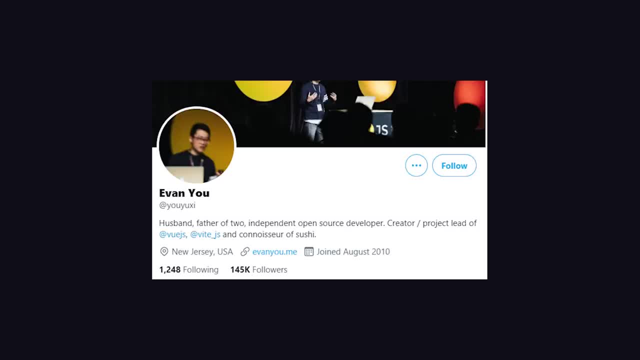 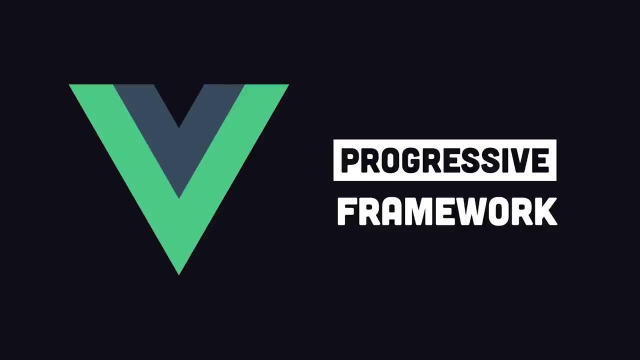 And that brings me to Vuejs, which is independently developed and maintained by Evan Yu and feels very similar to Angular, but in a package that's more approachable for independent developers. It has official packages for things like routing and state management and a huge ecosystem of third-party packages. It has the most: GitHub. 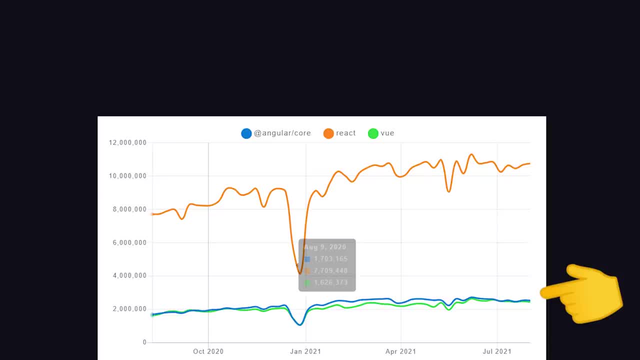 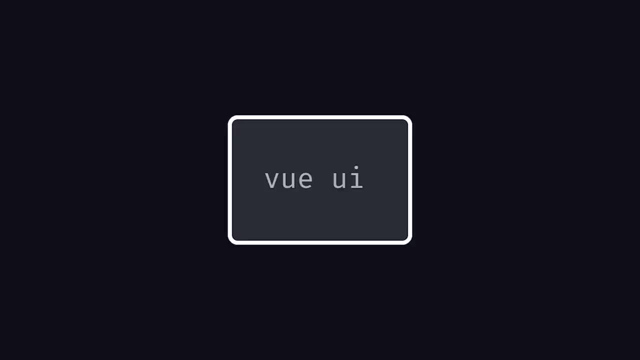 stars at 187,000 and is basically tied with Angular for second place on NPM downloads. Vue also has a very powerful CLI. For example, we can hit the Vue UI command which will bring up an actual browser window and walk us through all of the different dependencies. 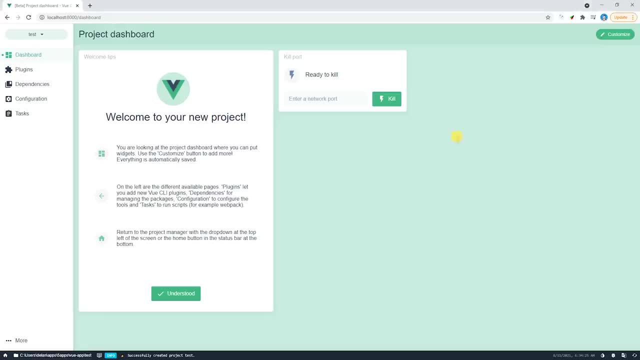 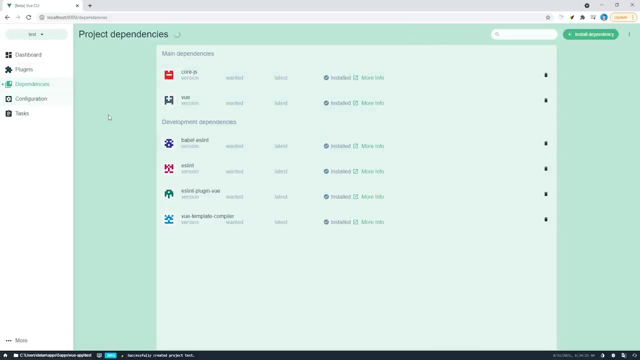 and features that we can add when generating the initial app. This creates a really nice developer experience, but it doesn't generate components and is just not quite as powerful as the Angular CLI. You'll notice it generates a far more simplified project structure, but in the mainjs file. 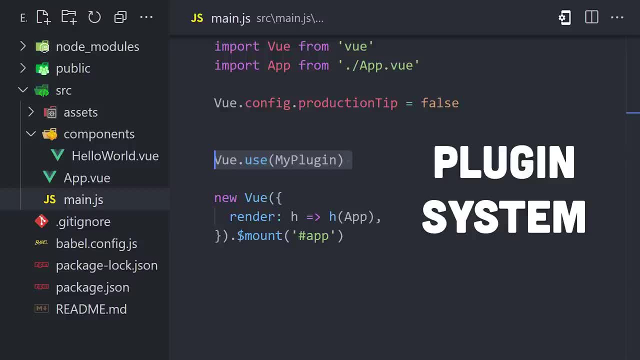 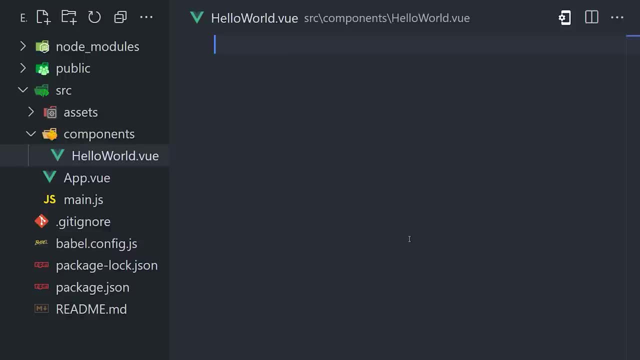 we can add additional plugins for other functionality like routing or state management, as it becomes needed. Components are defined in files that end in vue. The code is organized into three parts: a template, a script and the styles. The component itself is represented. 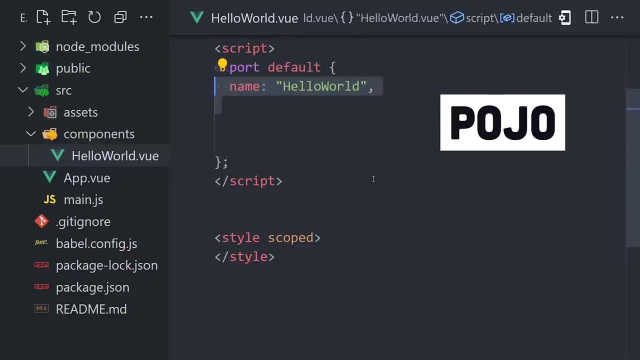 as a plain JavaScript object and we can define reactive data or state on it using the data property. Now to change the state, we have the methods property where we can define our add to do method that can be called when certain events are triggered. Then to tap: 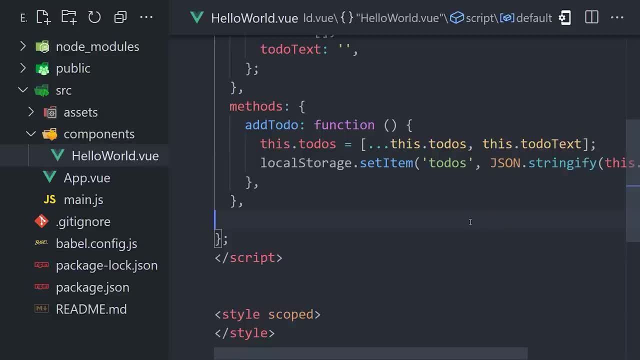 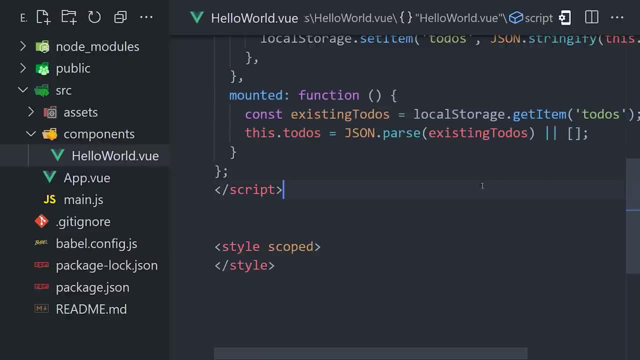 into the component lifecycle. we have methods like mounted- that will be called when the component is first initialized- Very similar concepts to React and Angular, the main difference being that we're working within the context of a plain JavaScript object instead of a function or class In the 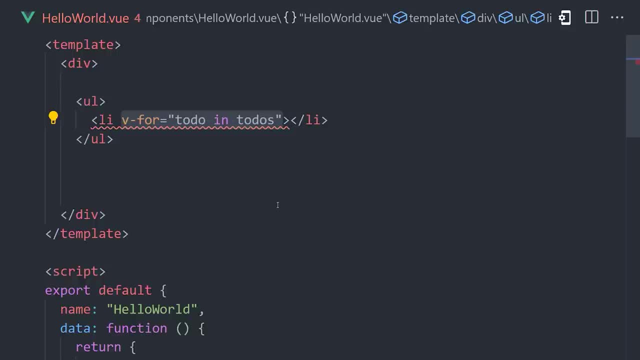 template. we have a setup that's very similar to Angular that uses directives to handle things like v for to loop over the to do items, or v on submit to handle the form submission. One thing that's nice here is that you can automatically prevent the default behavior by just adding prevent. 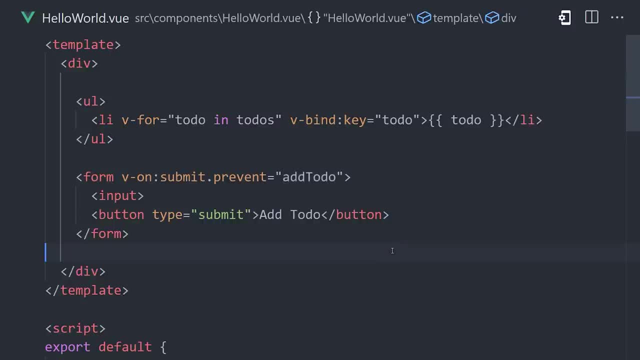 to this directive instead of implementing that code in the method itself. You'll find a lot of little things like that in Vue that make your life easier. And lastly, we have the v model directive to bind the to do text to the form input value. Vue is awesome and has a big community, but another 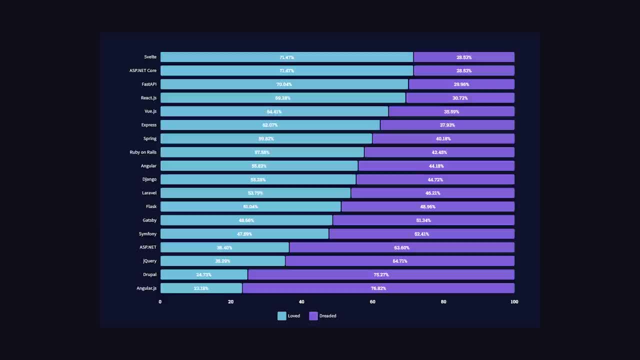 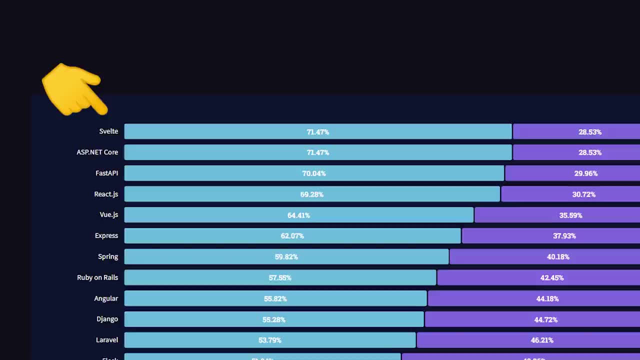 independent option is Svelte. It was the most loved framework on the 2021 Stack Overflow survey and has about 50,000 GitHub stars. It's not as common as the other three in the wild, but is very loved by the people who do use it. Like React, it's designed as a minimal library and relies on 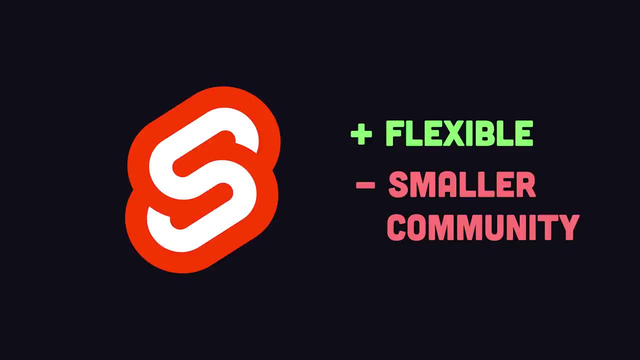 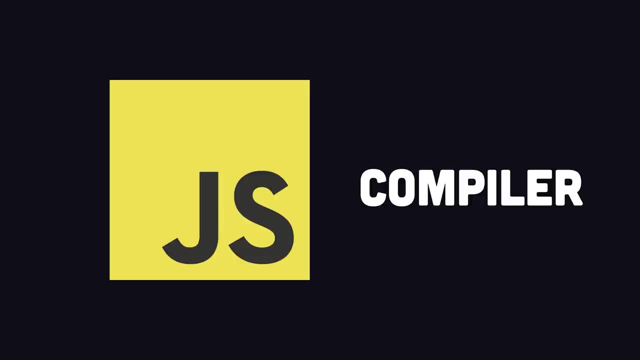 the open source community for other features like routing. One thing that makes it unique from the other frameworks is that it doesn't ship a runtime like virtual DOM to the browser. Instead, it works as a compiler to turn your code into plain JavaScript When you generate a new project. 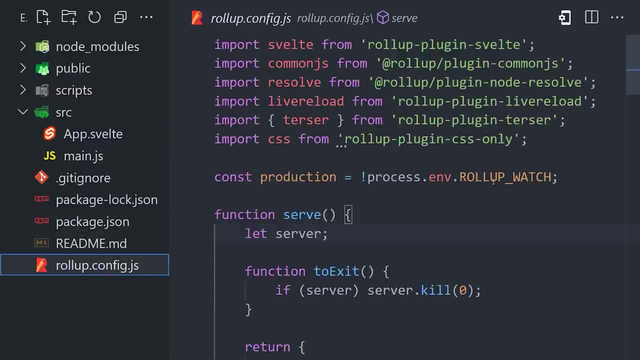 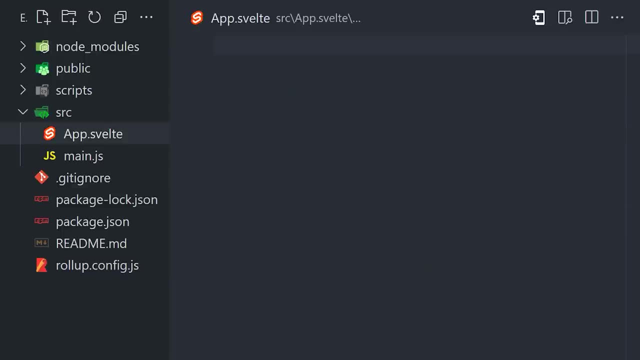 you'll have a rollup or webpack config if you choose, which is used to bundle your code, and all the other CLI tools attempt to abstract that part away from you. When building a Svelte project. you may need to learn a little bit about module. 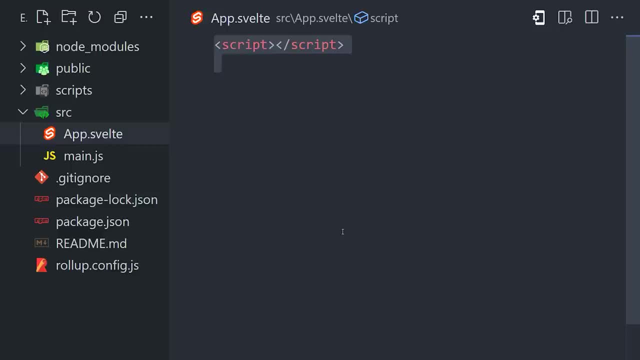 programmers, whereas the other frameworks try to hide that detail from you. Components are defined in svelte files and, just like Vue, they have three parts: the script, the template and the styles. To create reactive state on the component. just declare a variable with the let keyword. Then 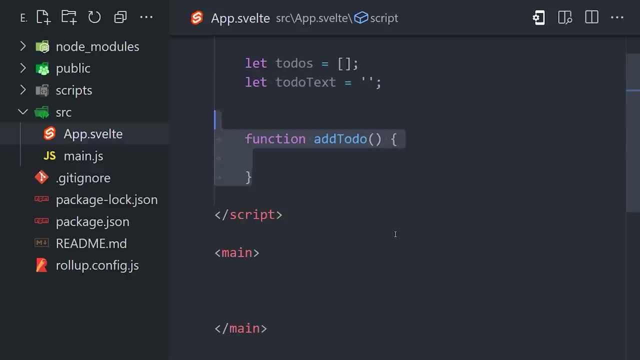 to modify the state, define a plain JavaScript function. What I like about this is that it feels very natural. It looks like regular JavaScript with minimal abstractions going on, compared to something like React. Now to deal with lifecycle hooks, we can import the onMount function from Svelte and register it as a svelte. Now, if we want to use the onMount function, we can import the onMount function from Svelte and register it as a svelte. Now, to deal with lifecycle hooks, we can import the onMount function from Svelte and register it as a svelte Now to deal with lifecycle hooks. we can import the onMount function from Svelte and register it as a svelte Now to deal with lifecycle hooks. we can import the onMount function from Svelte and register it as a svelte Now down in the. 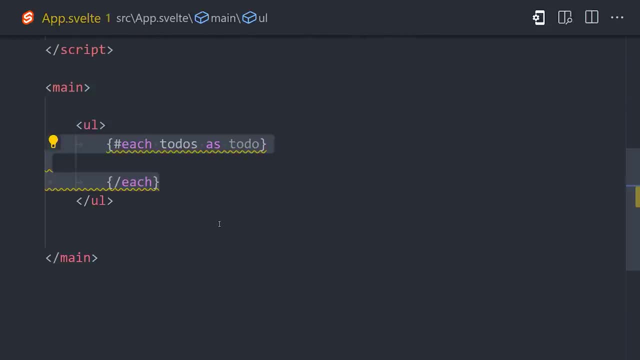 template. we have a special syntax that makes it easy to loop over things like each, to loop over each to-do in the array, Then to handle the form submission we have onButtonSubmit, and we can also add a bar with prevent default to avoid implementing that detail in the function. And lastly, we'll 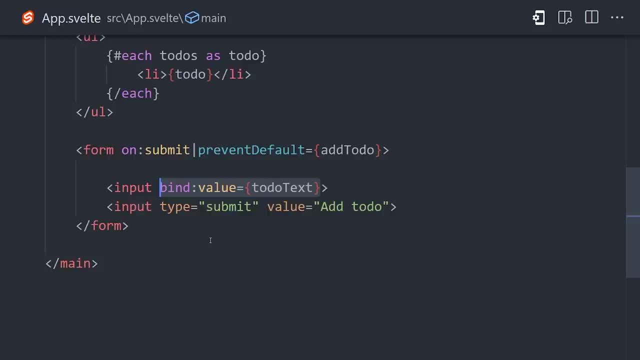 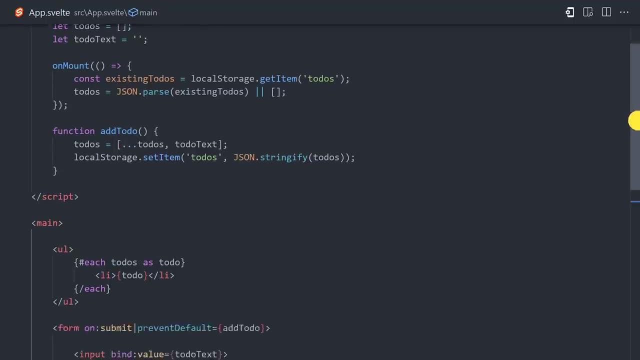 implement two-way data binding using the bind directive with value followed by the todoText variable. In my opinion, this is the cleanest implementation that we've looked at. It has the the fewest lines of code and it's fairly easy to read if you're a JavaScript developer. 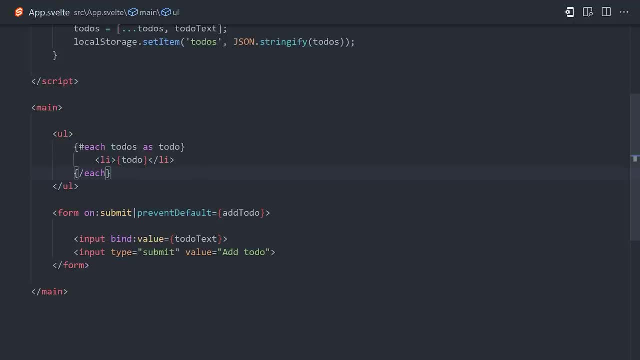 that has never used Svelte before. The drawback, though, is that the community is much smaller than something like React, So if you need to use a supporting library or if you're looking to get a job, you might run into some more roadblocks than if you used a more popular framework. 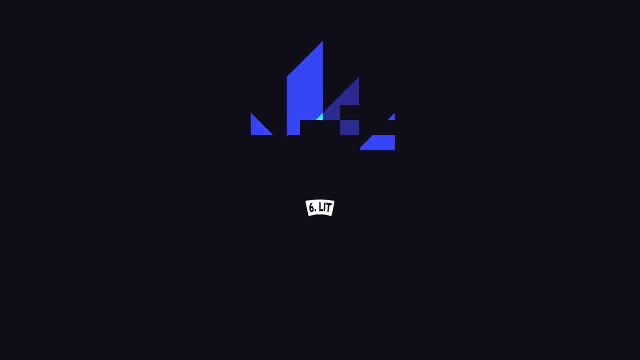 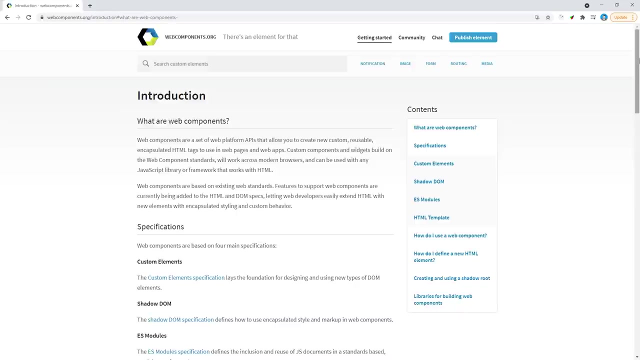 And the same goes for all the other frameworks that we'll look at from here, starting with Lit. Lit is a Google-sponsored project that's focused on building web components. If you're not familiar, web components are a browser standard that allows you to create. 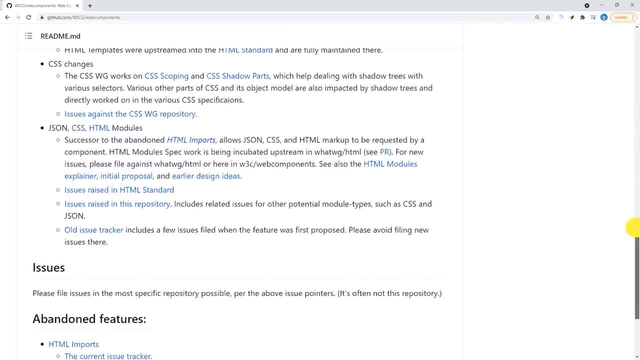 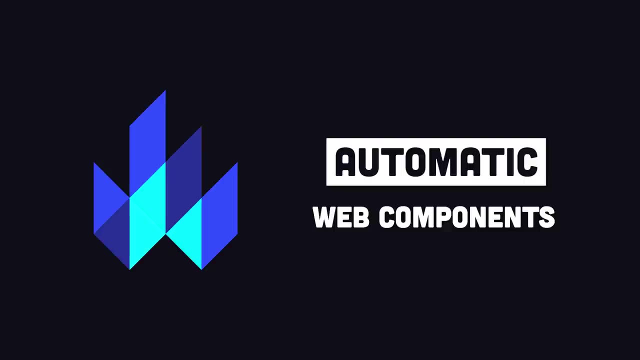 custom elements that can work across multiple frameworks Sounds great, but the Web Components API is notoriously difficult to work with. The cool thing about Lit is that when you define a component, it's creating a standard custom element under the hood. Now other frameworks can do that as well, but for most of them it's just an afterthought. 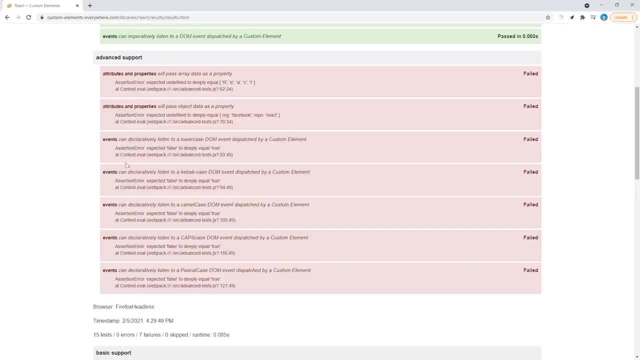 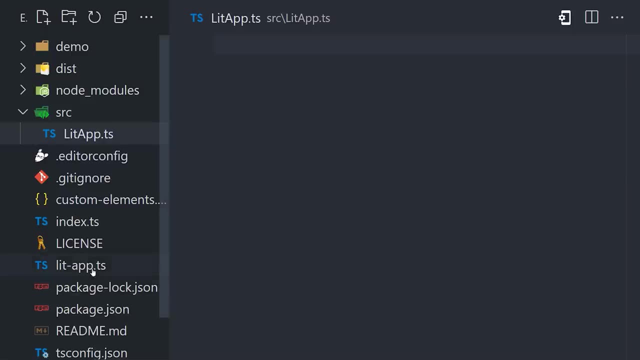 and the developer experience is usually not ideal if your goal is to build standard web components. Lit doesn't have a CLI of its own, but there is a starter project to get us going. I'm using the TypeScript version here, but that part is optional. 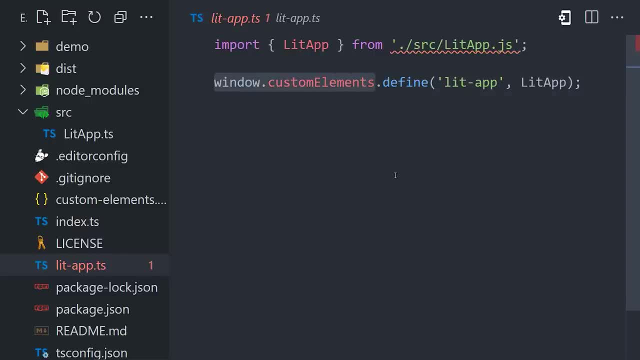 Inside the Lit appts file, you'll notice that it's calling windowcustomelements, which is part of the Web Components API in the browser. That's just a unique point that you won't see in other frameworks. by default, Components themselves are defined as a class that extends Lit element. 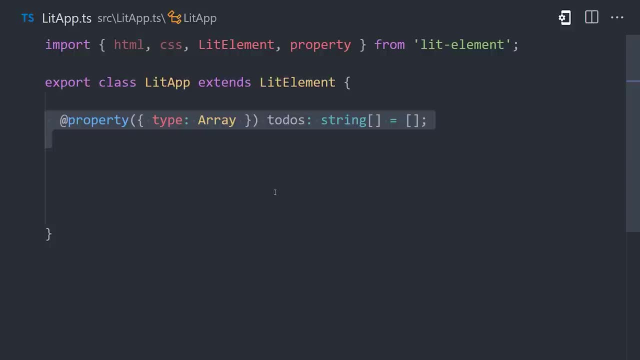 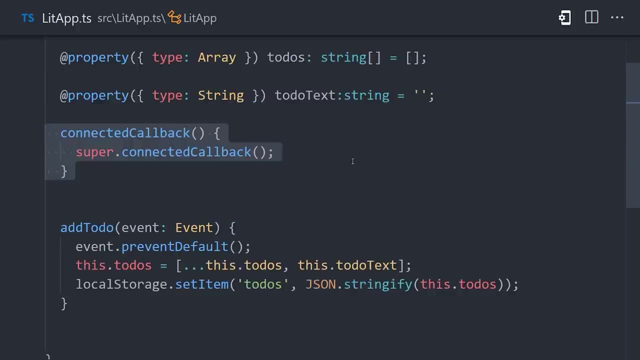 Reactive data can be defined as properties on the class using the property decorator. Then methods can be defined on the class to update the state Lifecycle. hooks are based on the ones defined in the actual Web Components API, like connected callback. By implementing the connected callback method, we can run code when the 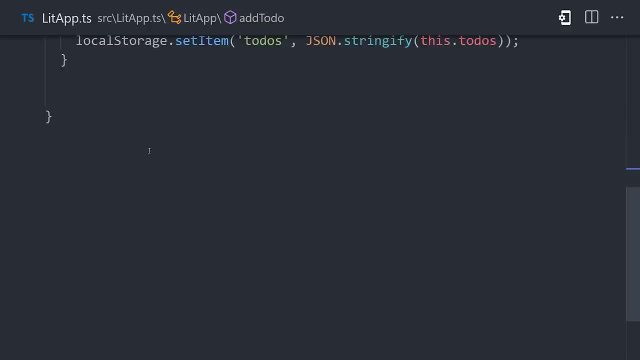 component is first initialized. Now, one thing that's really interesting about Lit is the way that it handles templates. It uses the existing template literals that we have in JavaScript, or in other words, a string that starts with backticks. This allows you to interpolate JavaScript into an HTML string using dollar sign braces. 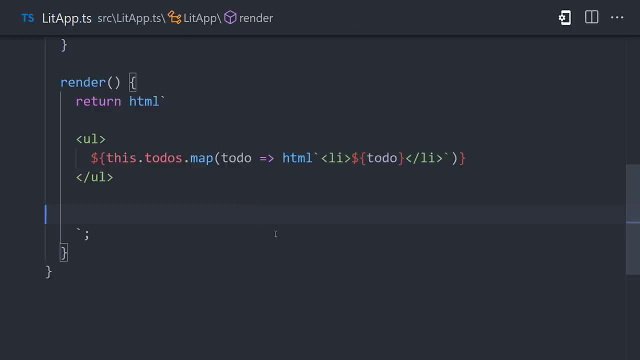 The end result is something that feels kind of similar to JSX and React, but the HTML can also have directives like submit or dot value to bind to the form, submit event or the input value, And, as far as I can go, I'm not sure if this is a good idea. 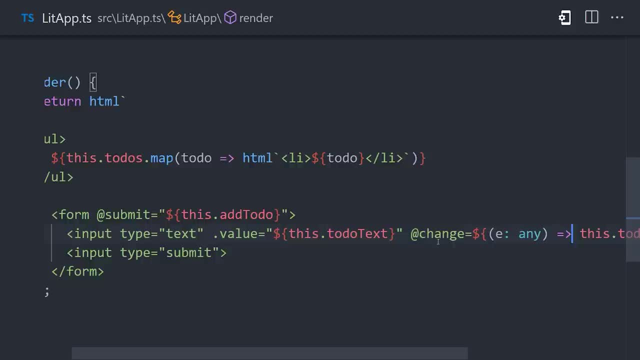 As far as I can tell, it doesn't support two-way data binding, so I had to set up an event listener here on the input change event to update the to-do text whenever that event fires. The bottom line with Lit is that you get a much nicer way to build standard Web Components without having to be an 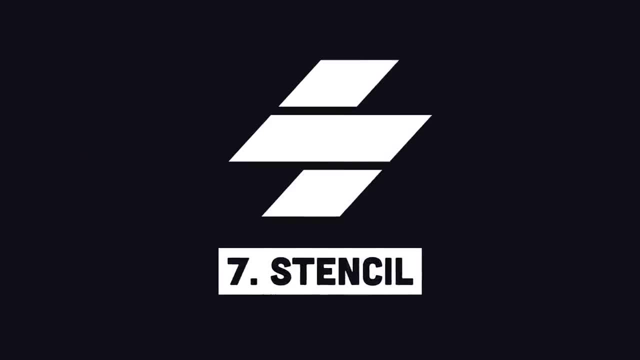 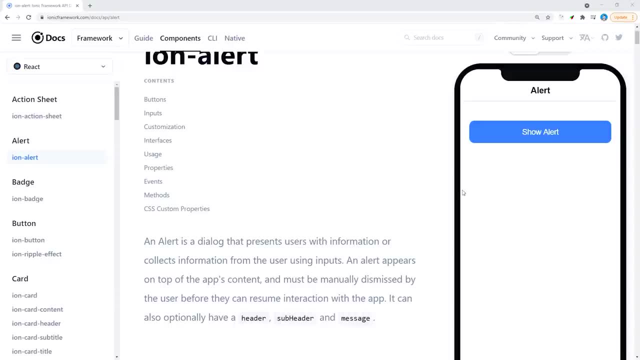 expert on the underlying APIs, And that brings me to an alternative framework that is also focused on Web Components, called Stencil. This one comes from the team behind the Ionic framework, which itself is actually a component library for mobile development that's built with Stencil. 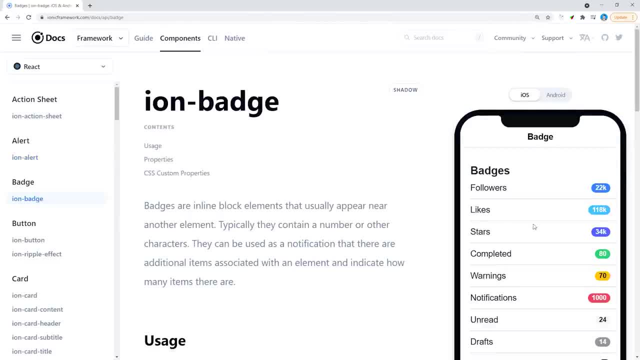 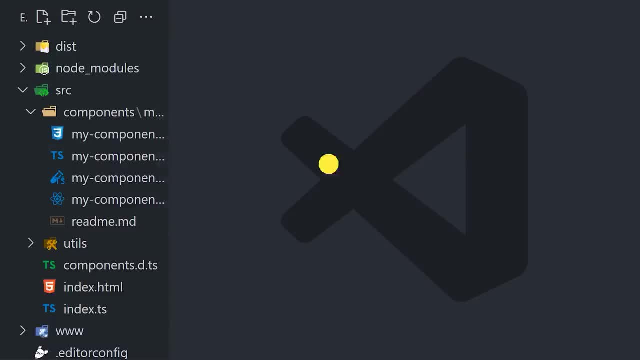 They use Web Components for the purpose of making applications more efficient, Making Ionic compatible with React, Angular and Vue out of the box. Create a new app by running npm init Stencil and that will give you a TypeScript project to get started. 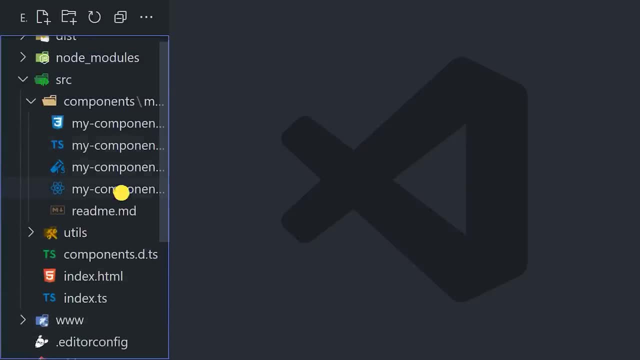 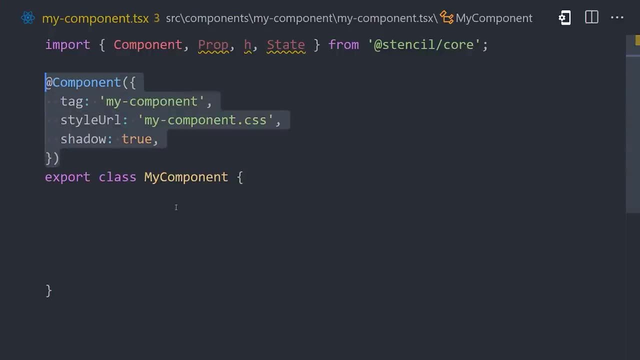 Just like Lit, it will take each component and compile it down to a standard Web Component. A component itself is a class with the component decorator which looks very similar to Angular. Then reactive data can be defined as properties. with the state decorator, Custom methods can be defined to update the state. 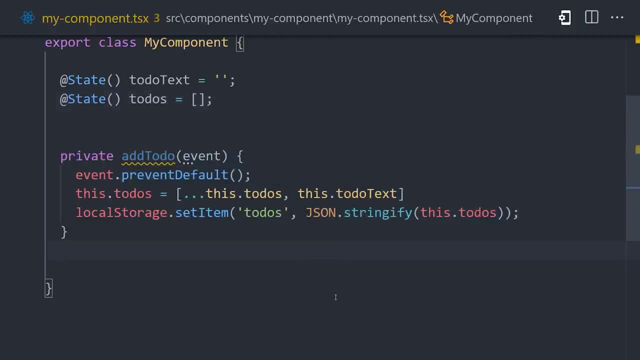 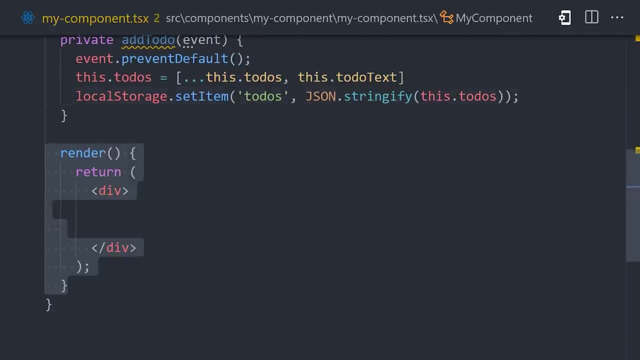 Then we have lifecycle hooks. like component will load to run code when the component is first initialized. At this point this component looks almost exactly like an Angular component, But for templating it uses JSX like React. That gives you the best or worst of both worlds, depending on who you ask. 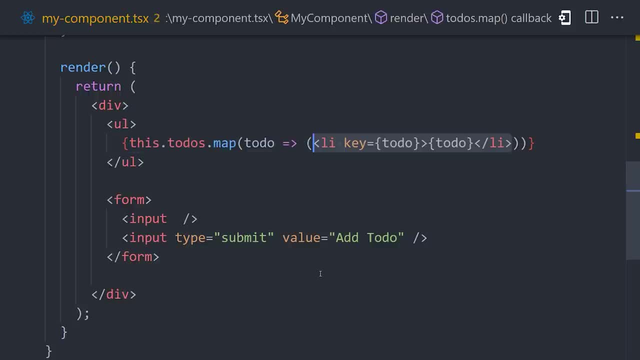 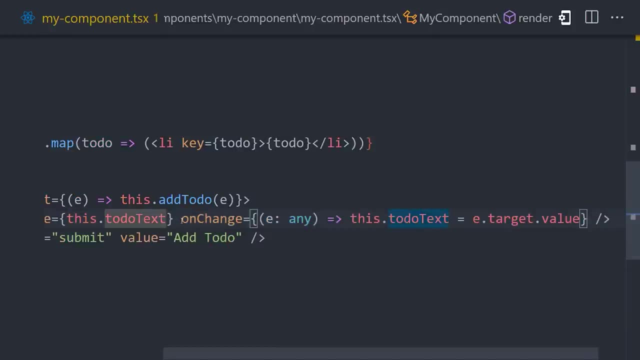 The template looks almost exactly like the React app, but it doesn't appear to support two way data binding, which means I've also added an extra event listener for on input to update that to do text when the user types into the form. Stencil is another great option for building Web Components. 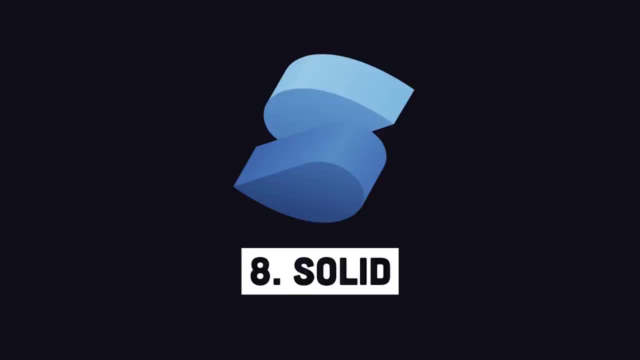 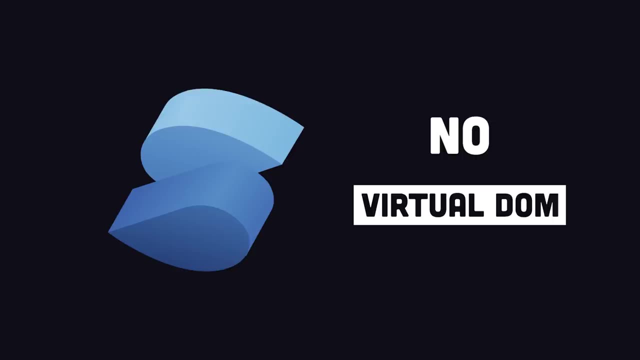 But now we're going to move on to a framework that I get a ton of requests for: SolidJS. It's a tool for building UI components and feels very inspired by React, but the main difference is that it doesn't use the virtual DOM. 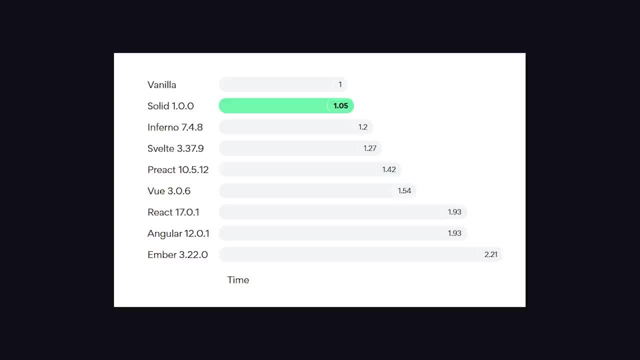 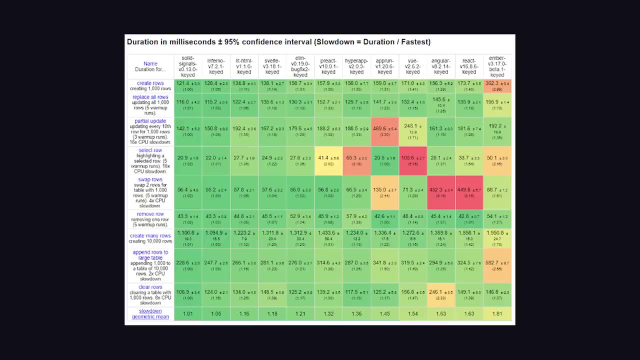 Instead, it compiles your code down to native DOM nodes similar to Svelte, And because of this it hits very high performance marks across every benchmark. You can think of it like a faster, more developer friendly version of React, but the drawback is that it has a smaller community to draw from. 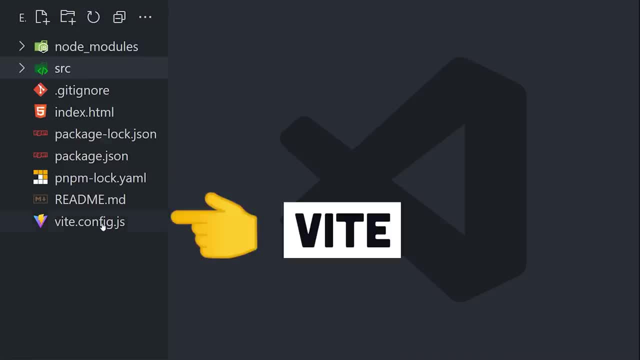 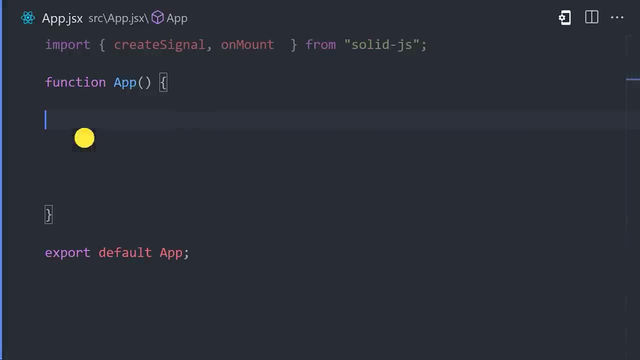 When you generate a new project, it uses Vite as the build tool, which is cool. Then you have components defined in JSX files, just like React. Then to define reactive state on the component, we use something very similar to a React hook called a signal. 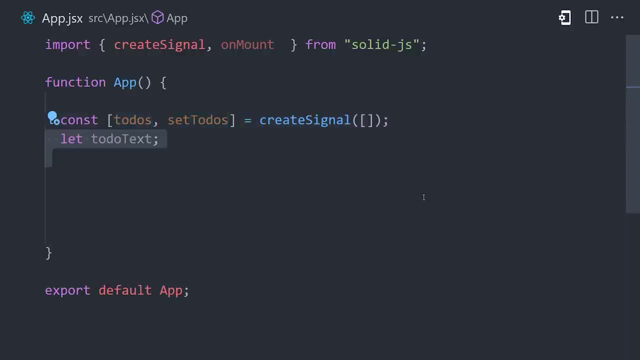 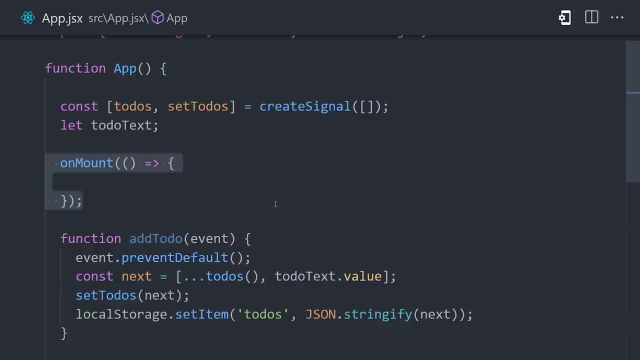 It returns us with a reactive value and a function to update that value. We can then define a function to update the state And if we want to use a lifecycle hook instead of use effect, we have the much more readable on mount hook that will run when the component is first initialized. 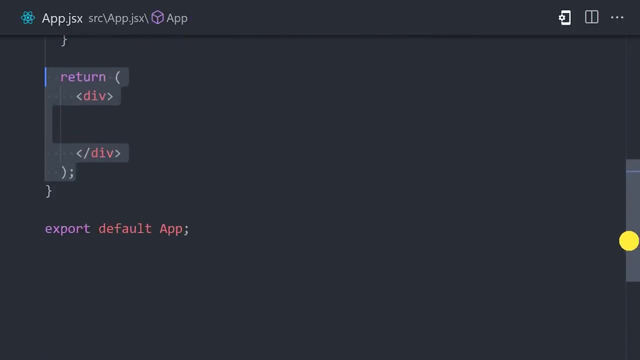 Now for the UI itself. we use JSX. It looks pretty much identical to the React code, but I've noticed that Solid does things to make your life easier. For example, we can Bind the form value to a variable using ref. 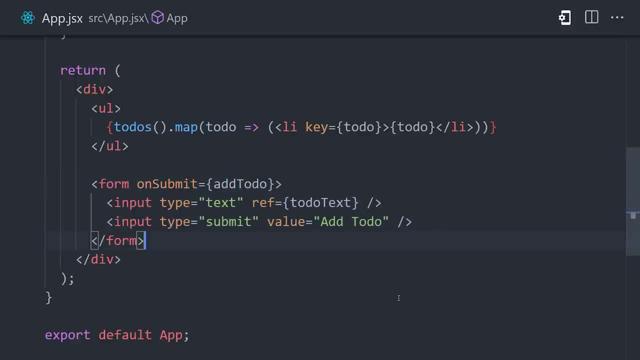 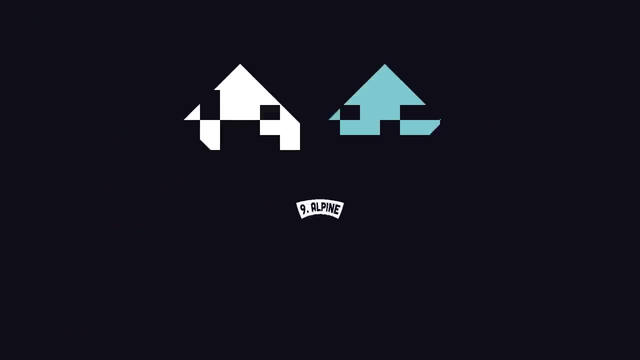 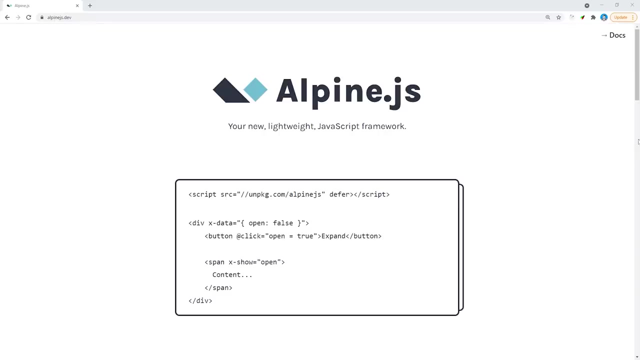 And, unlike React, we don't need to import the use ref hook to do that. Overall, Solid JS feels like a more well thought out and faster version of React. But now let's look at something totally different: Alpine JS. It's a tiny library at around four kilobytes that allows you to extend your existing HTML with reactive data and many of the features that you would find in the frameworks we've already looked at. 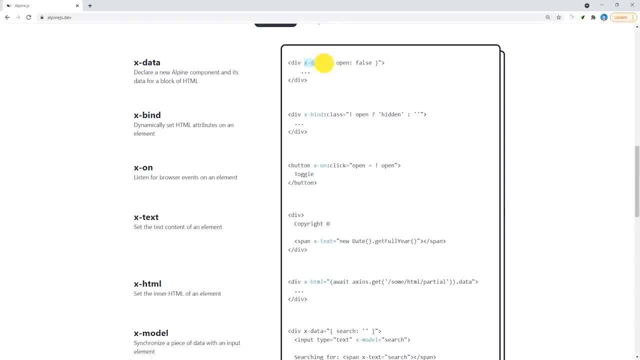 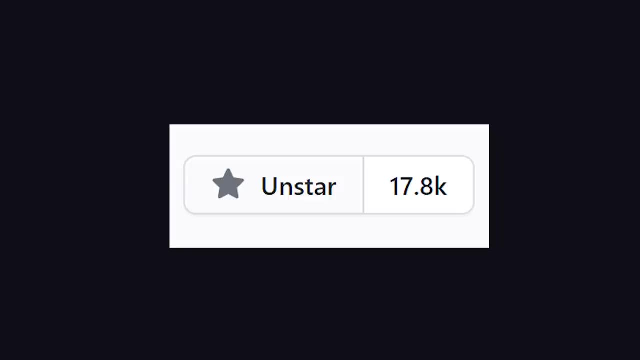 Instead of primarily focusing on JavaScript with Alpine, you generally focus on your HTML. If you've ever used Tailwind for CSS, you can think of Alpine as the equivalent in JavaScript. It has over 17,000 GitHub stars and is a popular replacement for jQuery. 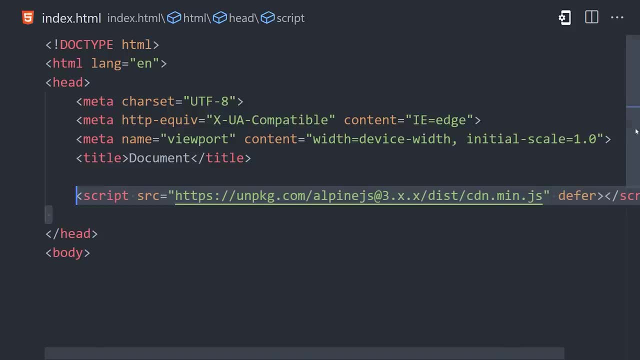 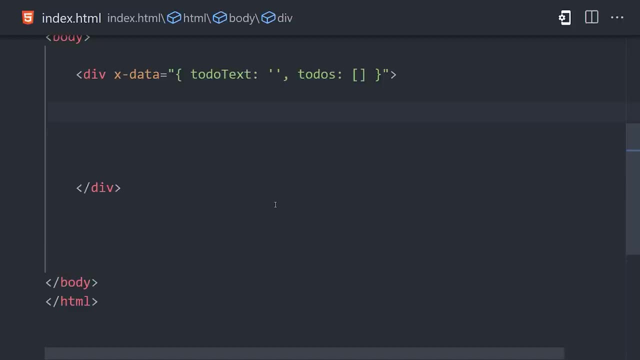 To get started, create an HTML file, then add the Alpine script to the head. Reactive data can be stored directly in a DOM node using the X data attribute. That data can then be used in a child element with something like X4 to loop over the array of to do's. 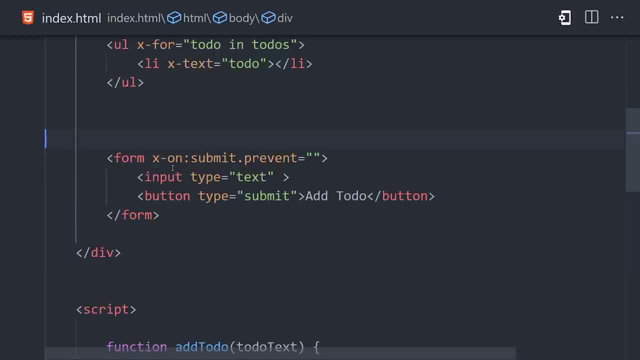 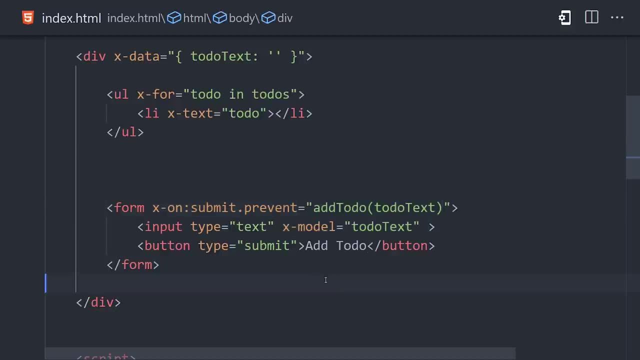 Then down in the form. we can use X on submit and also prevent default And then bind it to a variable, a function, in our JavaScript. The concepts here are very similar to the other frameworks that we've looked at, but in this case we're working with raw HTML, as opposed to some custom templating. 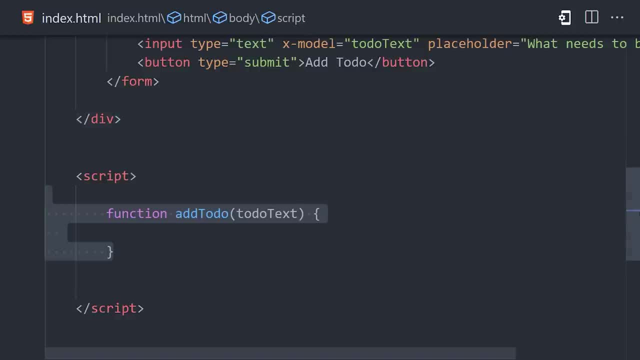 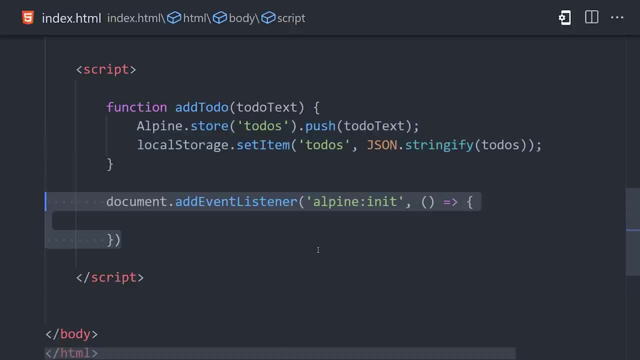 language or JSX. Now, if we do want to write some plain JavaScript, we can do that in a script tag, And Alpine actually has a mechanism called Alpine Store that allows us to store data and share it between multiple components in the UI. That's what we'll need to do for our to-dos, so that we can 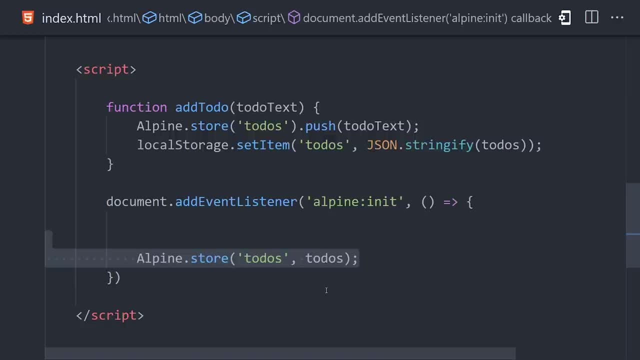 load them from local storage To handle that, when the component is first initialized, we can call document, add event listener to the custom Alpine init event and then update the data from the store when that event fires And that gives us a complete app with very minimal code, In my opinion. Alpine. 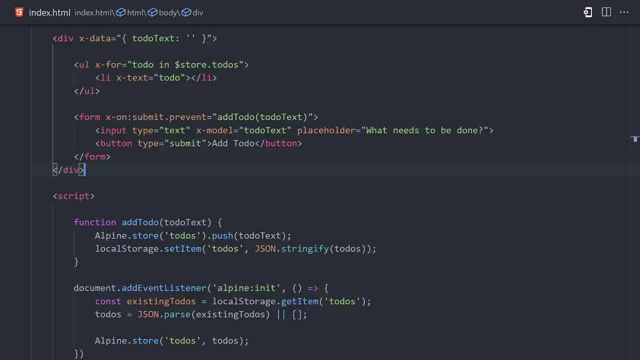 feels like an awesome option when you just want to add a little bit of JavaScript interactivity to an existing HTML page, But at the same time, I don't think Alpine could replace something like React, Vue or Angular. So if you're building a very complicated single page application, it might. 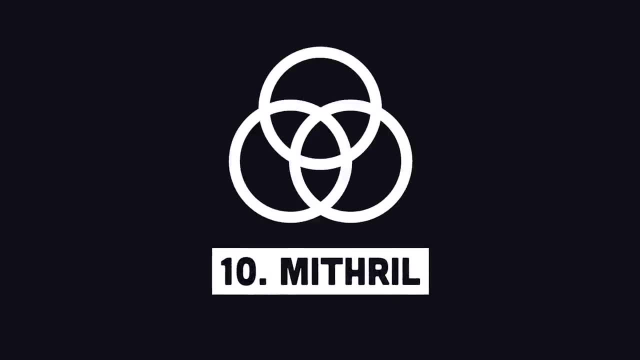 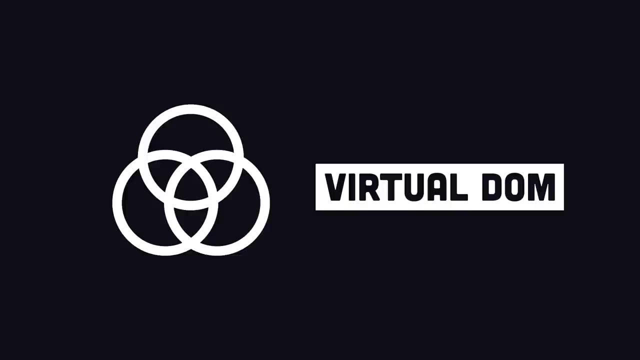 be best to stick with one of those. And that brings us to the final wildcard framework, Mithril. It's also very lightweight and tends to perform better than the big frameworks. It uses virtual DOM like React and Vue, but the overall developer experience is a lot different. To get started, create an index. 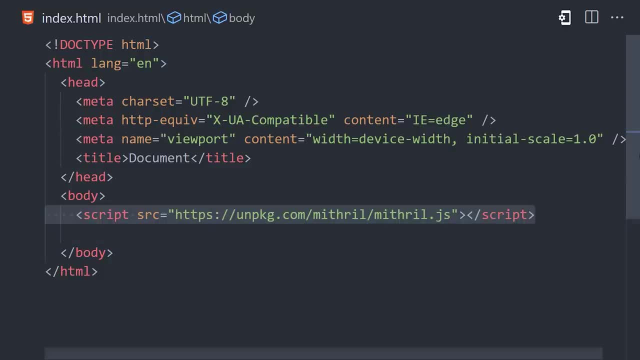 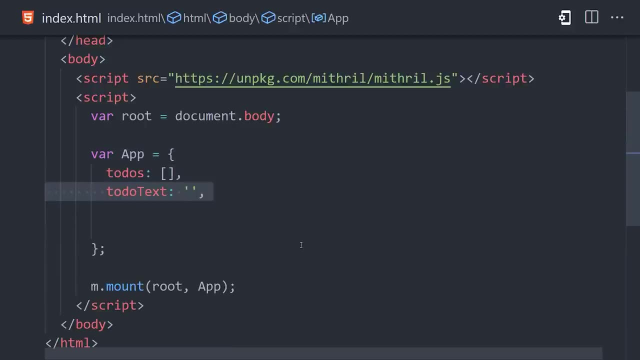 HTML file, then add the Mithril script tag to it. You can actually create components from functions, classes or, as we're doing here, a plain JavaScript object. We can add data and methods to the component as properties on the object. There are also special properties, like on init, which is: 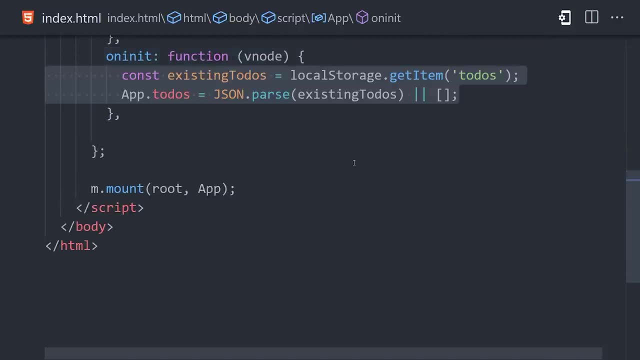 the lifecycle hook for when the component is first initialized. Then we have Vue to define the UI itself. To define a DOM node, we use the M function and pass the name of that node as the first argument, then options about the node as the second argument, like the class name. 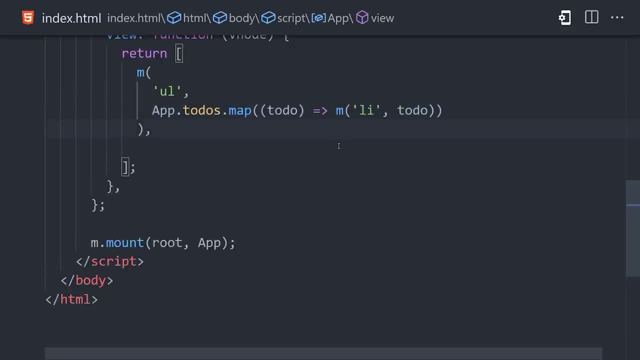 for example. Or you can pass children as the second argument, like we're doing here, to map an array of list items. Then, down on the form element, we're defining a handler for the on submit event. What you have here is something that is kind of similar to JSX, but the UI is truly. 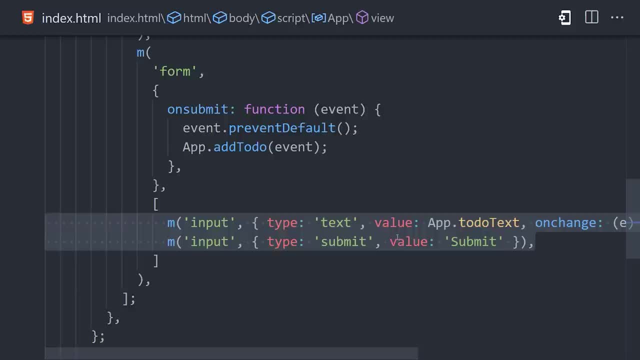 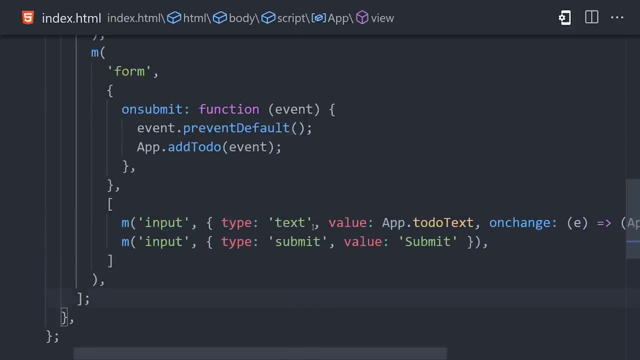 defined in pure JavaScript. If you hate HTML and never want to touch it, you might like this system, But personally I found it a bit awkward and the Mithril app actually took me the longest amount of time to build. But, like I said before, it really comes down to personal preference and I